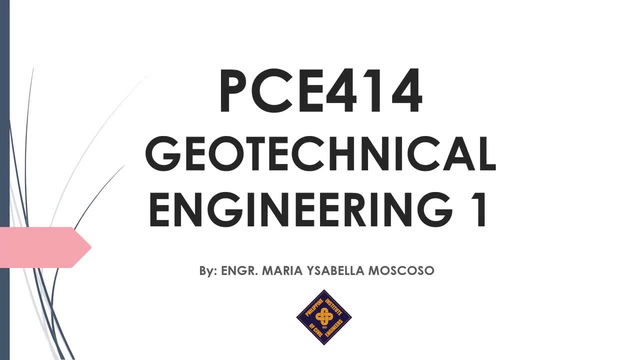 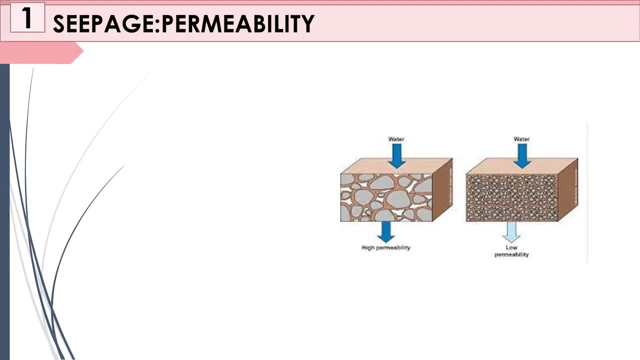 Hello, good day everyone. So welcome back to our PC414- Geotechnical Engineering 1.. So we will have another topic for this morning or for this day, and our topic to be discussed is all about permeability. Okay, so before we start, let us start to define what is permeability? 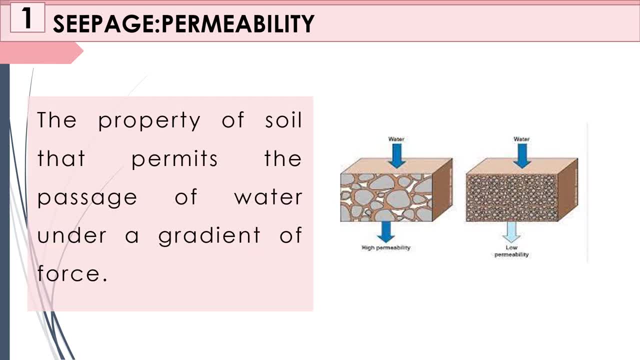 is all about. So, according to this one, permeability is the property of soil that permits the passage of water under a gradient of force. Okay, so in simplest explanation, what is permeability is all about? Okay, permeability is the movement of a fluid. 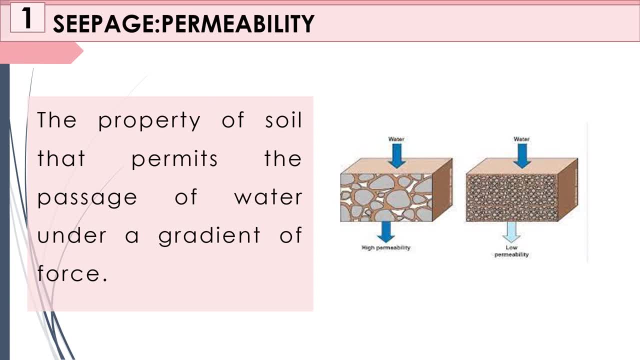 through soil. So meaning to say hindi lang pala naglalak sa idea na tubig lang yung pwede Any fluid that pass through the soil. That is why, kung naalala ninyo on our previous topic, yung aking example is that when yung water is tinapon, natin sa soil. 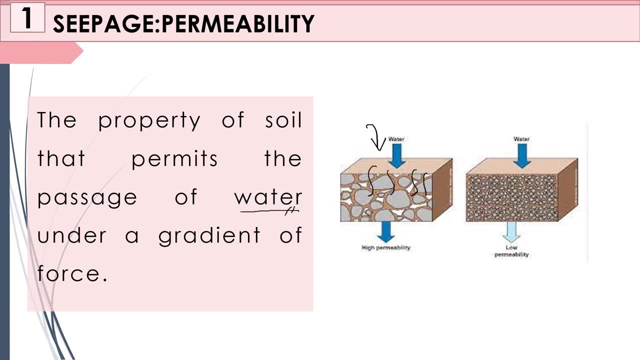 okay, nawawala yung soil sa ground, pumapasok siya sa lupa, It's because of permeability. Okay, so, going back on our first topic during the prelims di ba soil classification. now we know that our soil is composed of solid soil particles, where meron tayong tinatawag na. 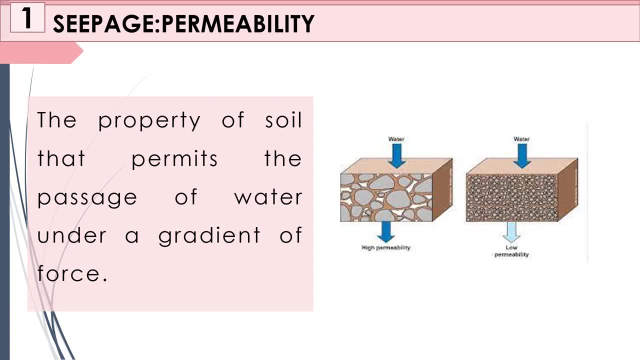 voids. okay, Going back to our soil constituents, sabi natin dito that our voids is composed of air and water. okay, So, because of these voids, now, dahil sa voids na ito, our soil or the soil allows or permit the fluid to pass through the soil mismo. Okay, because of the vois kaya nakakapasok. And because of the voids, so it's inviolable. it really nationalizes whichboil comes from and that's not true. okay, I'm used to it. I know that we're doing interview, like we're using exposure to soil and what it's like being in it. I know I'm not so familiar with it so I don't know that many people learn technique. 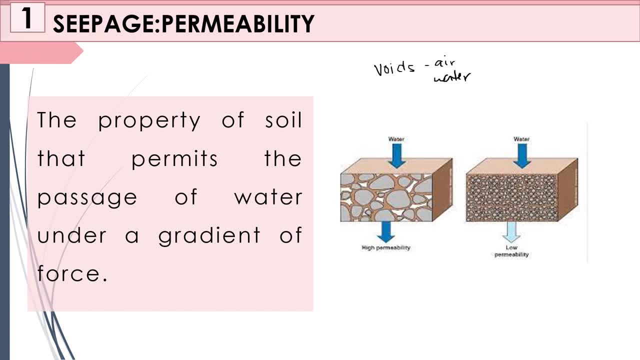 because of the voids, kaya nakakapasok ang�wala at leadsh iが ang contabilidad sa solidity or естеeng stress. okay, yung fluid natin sa ating soil, So ganito na lang. 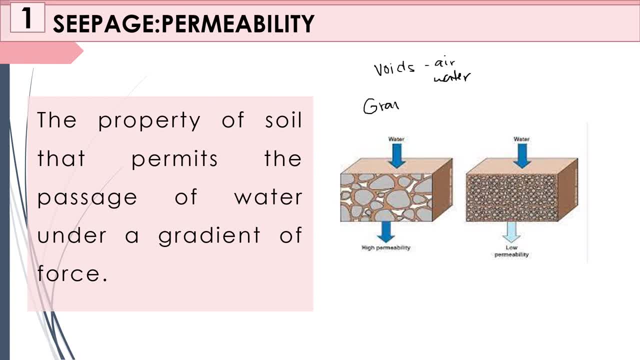 isipin natin, For example: here we have the gravel. Okay, Kapag gravel yung soil particles natin, we know that the void present in that soil is bigger. So sabihin natin na yung 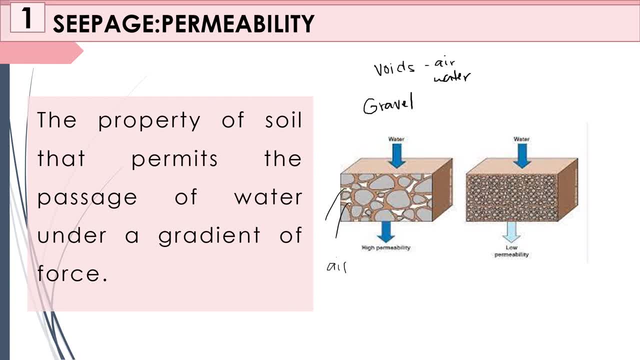 voids. dito is air Okay, Sobrang laki ng volume ng air dito. So pag tinaponan natin to ng tubig, anong mangyayari? Saan ba pupunta yung tubig Matik? no, Basically. 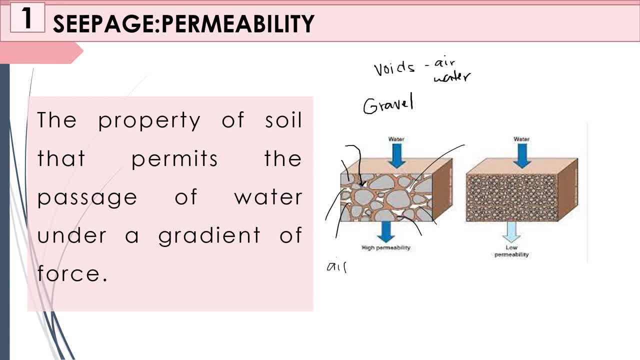 yung tubig ninyo is papasok siya, kung nasa ang merong space na pwede, Where Yung voids na tinatawag natin Okay, And because of that voids nagkakaroon din tayo ng. 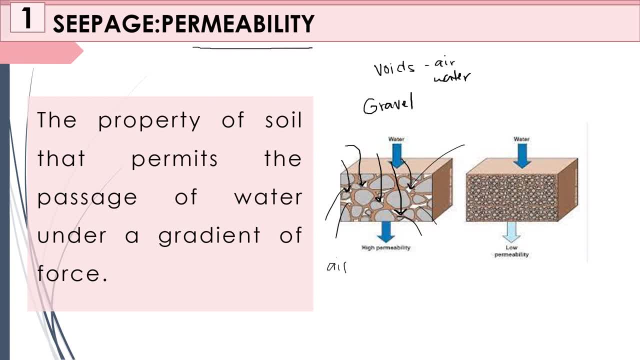 permeability. Okay. So ibig sabihin no, the bigger the volume of the voids? no, like, for example, the gravel, it has the high permeability, It has the permeable soil. Ibig sabihin mas malaki. 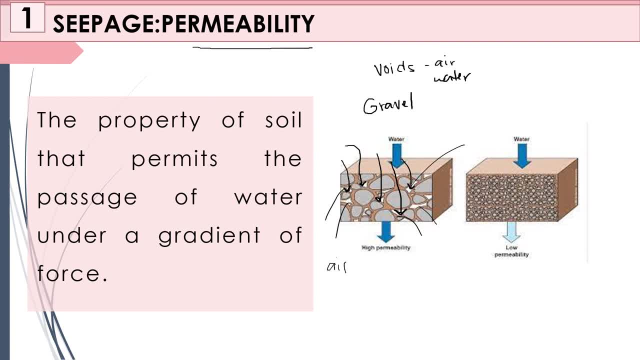 I mean mas mabilis yung pag-permit ng fluid natin sa soil, Where, kung iko-compare naman natin yung gravel to clay, okay, as you can see, no clay has a smaller volume of voids. 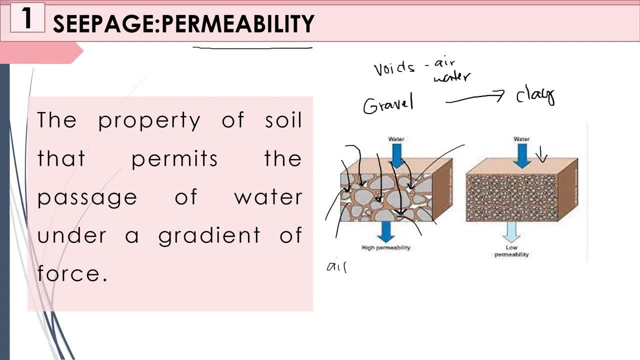 Ibig sabihin, kung bubuhusan natin to ng tubig, hindi agad papasok yung tubig sa clay. Now it's because its composition is compacted. Halos wala na tayong makita. 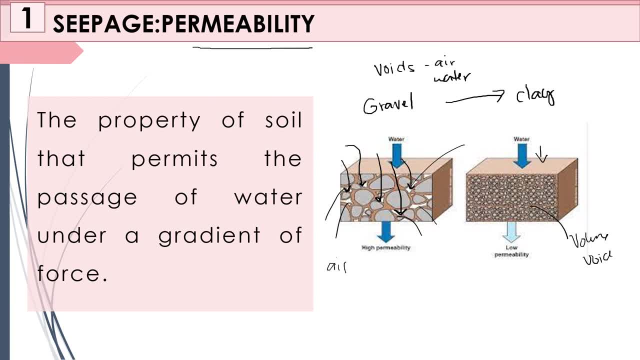 na volume of your voids? No, pero meron pa rin yung papasok. No, pero konti lang. So ibig sabihin it has a low permeability. So that is the difference. no, 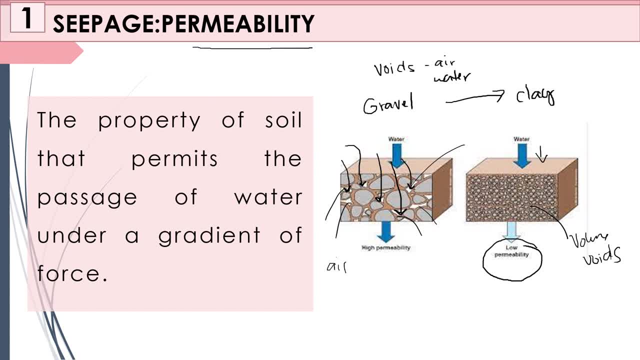 when the soil particle has a bigger void or bigger void volume, ibig sabihin it has a high permeability, While no soil has a lesser or smaller volume of the voids, meaning to say it has a low permeability. 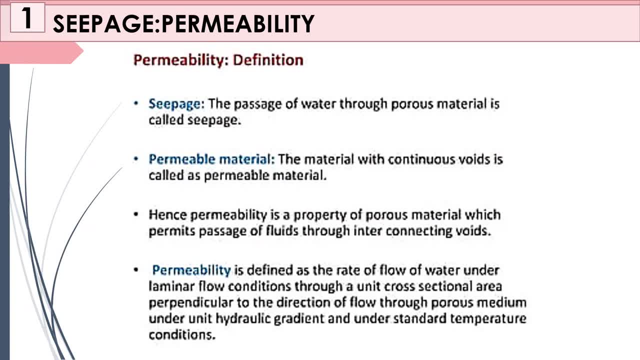 Sana nuggets yan. Okay. So dito naman let us try to define permeability. So simulan natin from the word seepage. Okay, Ano ba yung ibig sabihin ng seepage? 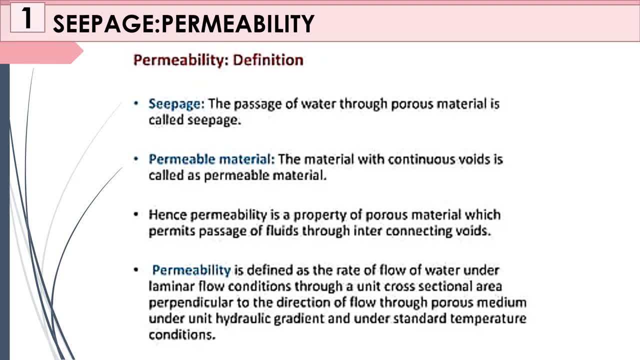 O ito yun. Seepage is the passage of water through porous material. Okay Again, seepage is the passage of water or fluid through a porous material, While permeable material is the material with continuous void and it is called. 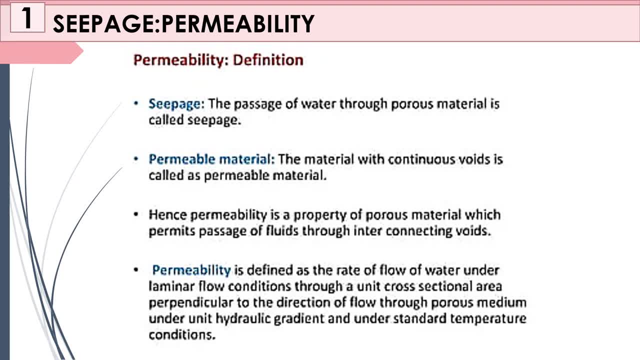 permeable material: Okay, Ito na. So when we see permeability, no, since it is a property. so let us try to define this as the rate of flow of water under laminar flow conditions. Okay, Through a unit cross-section. 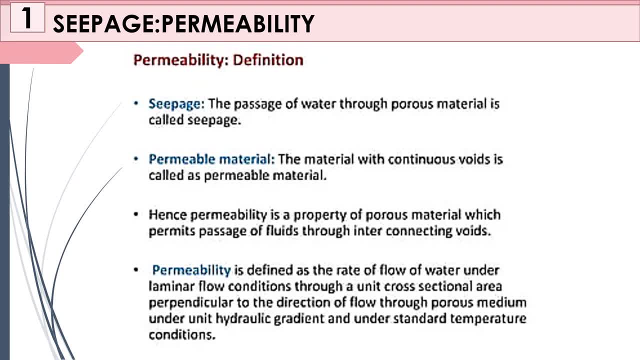 area perpendicular to the direction of the flow through porous medium unit hydraulic region and under a standard temperature conditions. So meaning to say, pag pinag-uusapan natin yung permeability, we are considering a laminar flow condition. Okay Kasi, kapag 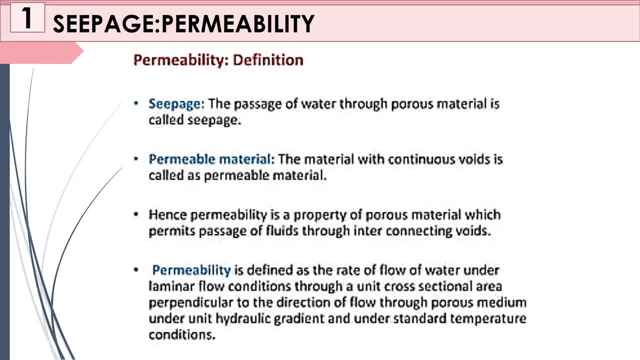 nag-consider na tayo ng turbulent flow o yung soil natin baka kumunoy na yun or quicksand. Okay, So yung pag-permit ng tubig natin or yung pag-permit 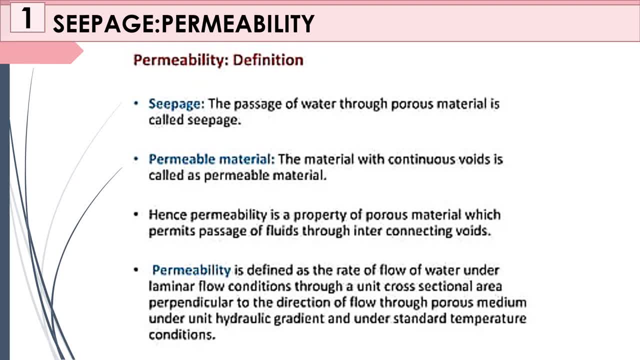 ng fluid natin through a porous material, which is most commonly soil, yung tinatawag natin yun the rate of flow. no, ng pagpasok ng fluid natin sa ating soil is tatawagin natin yung. 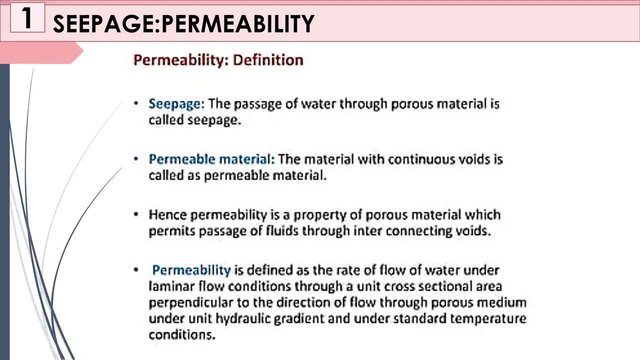 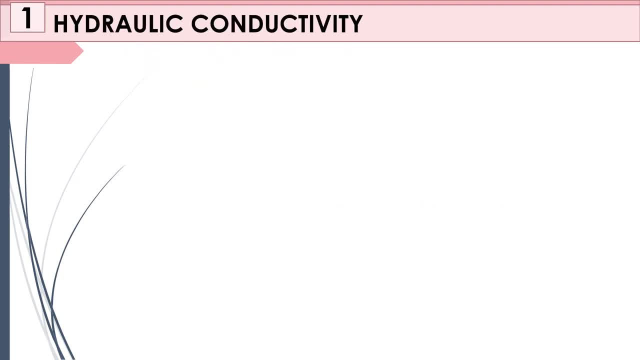 permeability Or permeability, And take note again: no, ang pinag-uusapan natin dito is a laminar flow. Okay, So pag-uusapan naman natin yung mga components kapag pinag-uusapan. 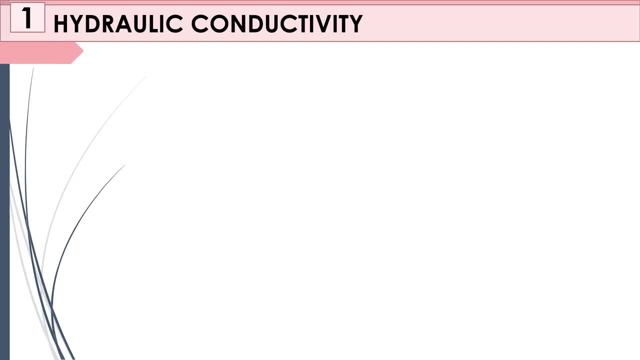 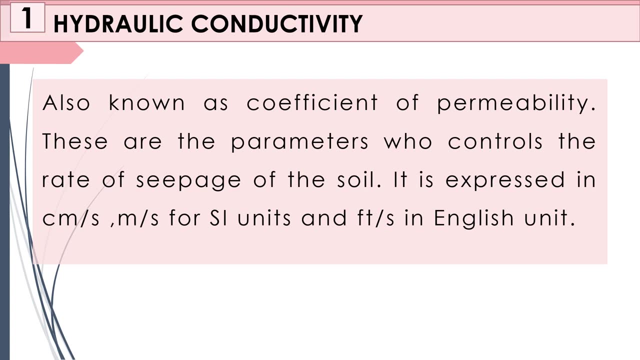 natin yung permeability, And first thing is your hydraulic conductivity. So what is your hydraulic conductivity? No, it can also be called as your coefficient of permeability. These are the parameters. who controls the rate of seepage of the 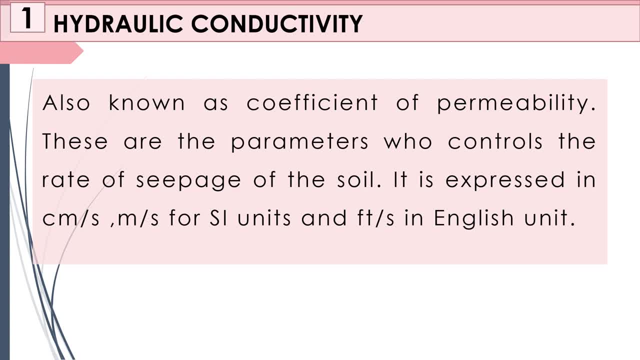 soil. It is expressed in centimeter per seconds, meter per seconds for SI unit, or it could also be feet per seconds in English unit. So nagets ba by the definition. So ibig sabihin: your coefficient of permeability. 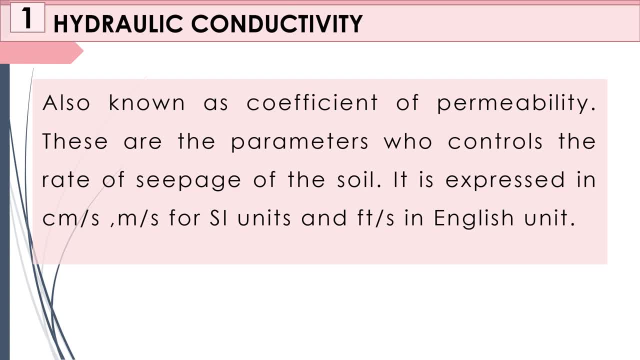 or your hydraulic conductivity? no, yan yung magiging parameters natin to control the rate of seepage of the soil. Again, what is seepage? No, yan yung pag-permit or yung pagpasok ng ating water. 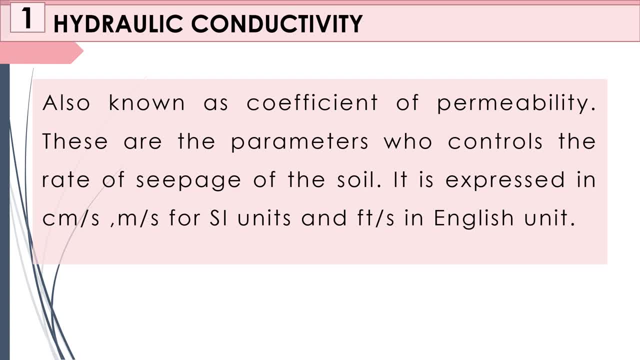 into a porous material. So itong hydraulic conductivity natin, no, aside from being its parameter, so yung hydraulic conductivity natin is nakadimitro- depende din sa pagka-viscous ng material. Okay, Because we all know that ano ba yung viscosity? 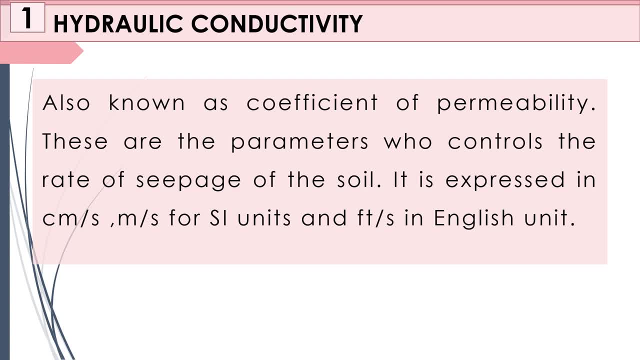 No, going back to hydraulics. So yung viscosity that is the resistance of the fluid diba to flow. So ibig sabihin, kapag mas malagkit yung ating fluid, mas viscous yun. 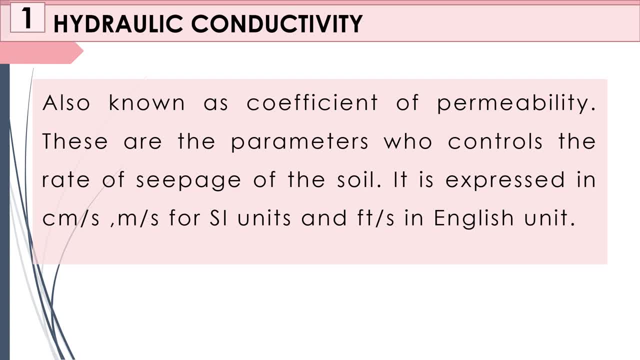 Mas mahirap yung kanyang pagflow. Okay. So ibig sabihin, kapag less viscous yung, mas material, mas mabilis yung flow natin. That is why for this topic, 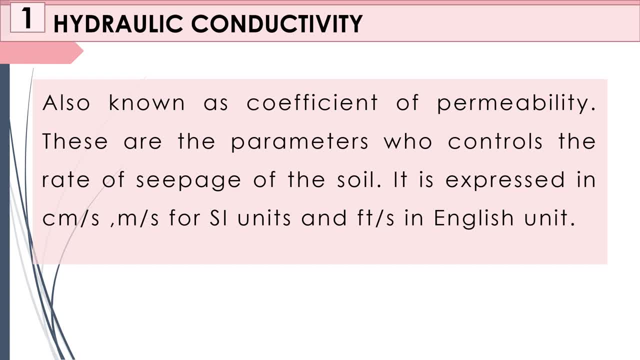 kinukonsider natin yung tubig? no, kasi less viscous sya. And aside from the viscosity of the fluid, no, when we're talking about hydraulic conductivity, tinitingnan din natin yung pore size distribution. 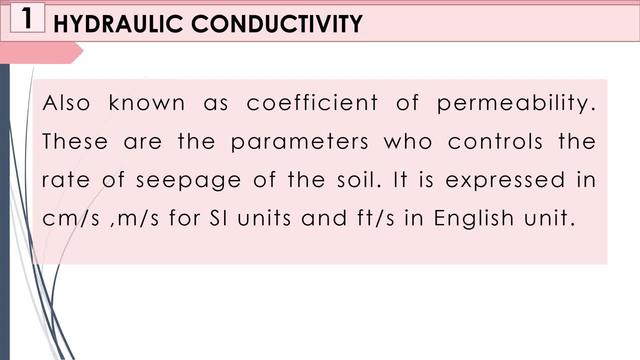 which is yung soil particles natin And as well as your voids. no, it's because nakadepende nga sa voids yung magiging permeability. Parang ano ba ito permeability status ng ating soil, if that is? 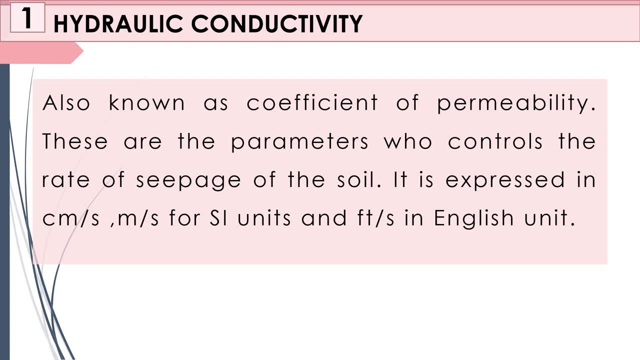 high or low permeability. Okay, So, talking about viscosity, okay, so going back to your hydraulics, we know that your unit weight and your viscosity changes with respect to the temperature. Ibig sabihin linear to Kapag nagbabago. 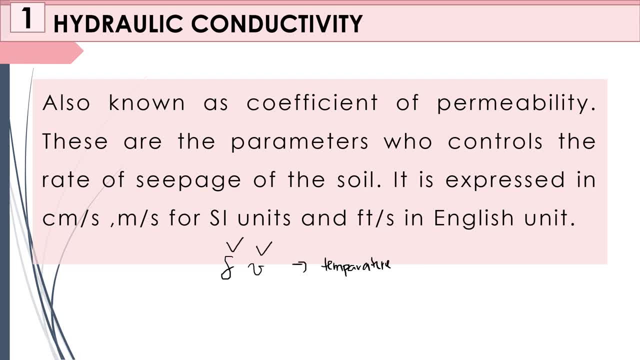 yung temperature nagbabago bago din yung value ng unit weight at ng viscosity. That is why, naalala ninyo, kapag 4 degrees and 20 degrees iba yung value ng unit weight of water as well as. 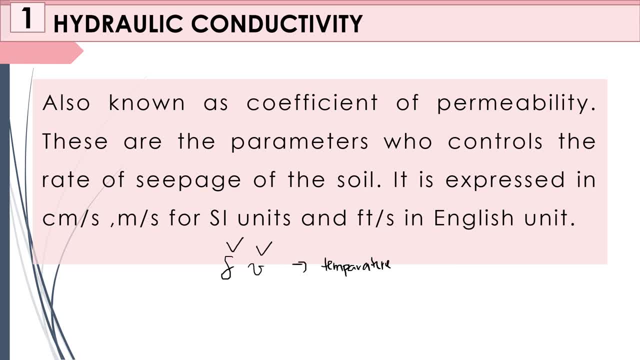 for the mass density? no, because that is because of the temperature. So when the temperature changes, your unit weight and the viscosity also changes. So ganun din yung hydraulic conductivity. When the temperature changes, your hydraulic conductivity also changes. 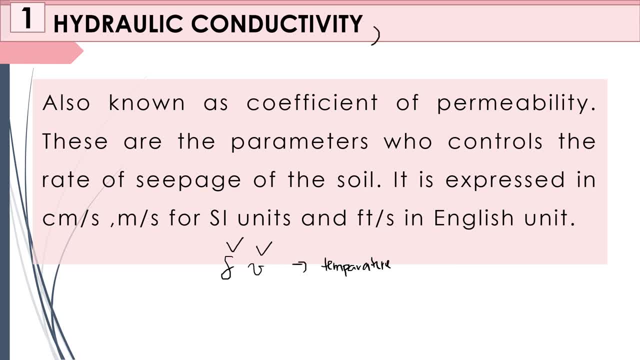 Okay, And hindi ko pala nasabi kanina na, that the variable for your hydraulic conductivity is, tatawagin natin, tong variable K. Okay. Okay, So to express na no, para maging uniform tayo sa ating solution. 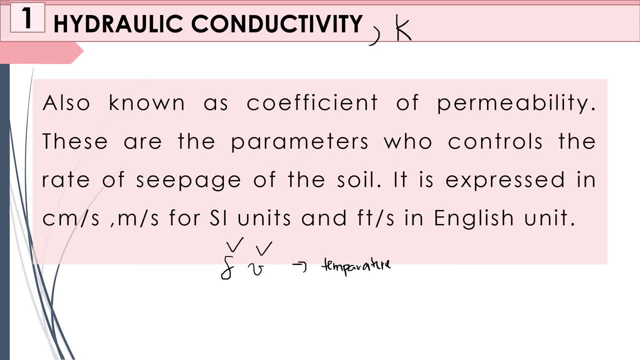 so let us say na that the standard temperature kapag pinag- uusapan natin yung hydraulic conductivity, that is in the temperature of 20 degrees Celsius. Again, K is your hydraulic conductivity, or your coefficient of permeability, And that is expressed in meters. 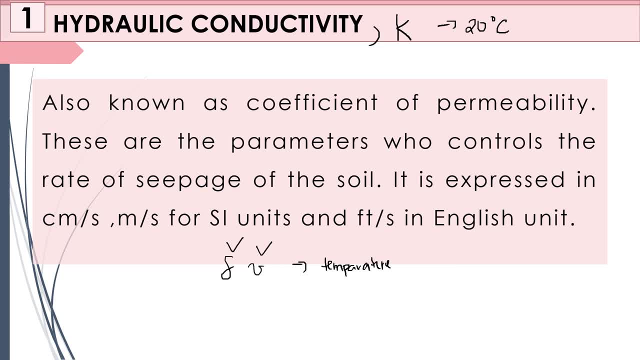 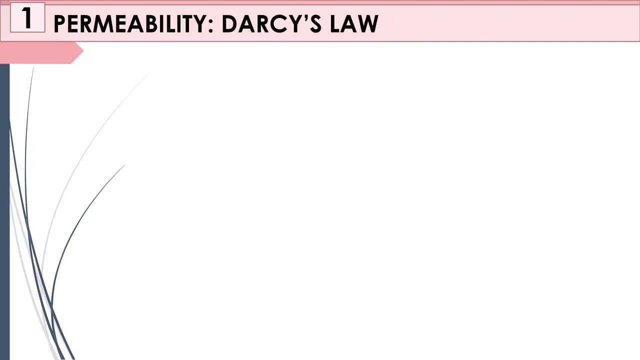 per seconds. No, parang velocity, Which is makes sense, no, Which minimesure natin yung flow rate, no, ng pagpasok ng fluid natin sa soil. So moving on to our Darcy's Law, 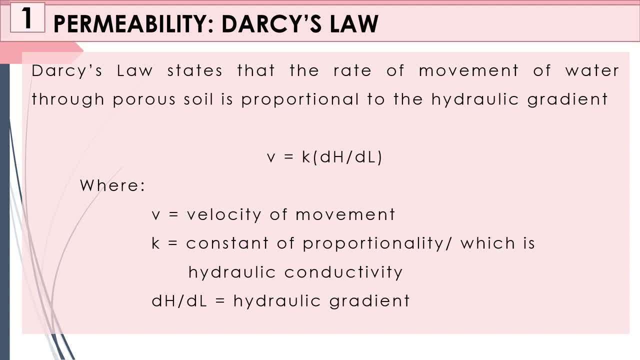 no formula naman ito. So Darcy's Law states that the rate of the movement of the water through a porous soil is proportional to the hydraulic gradient. So you have the formula here of: V is equals to K times DH over DL. 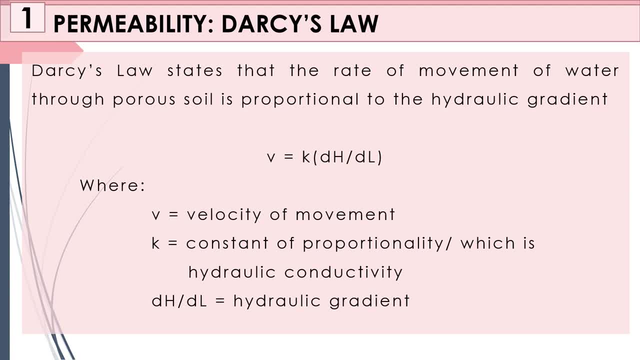 Where V is the velocity of the movement and K yung bago nyo lang nakilala kanina, which is your coefficient of permeability, or your hydraulic conductivity, And your DH over DL. there is your hydraulic gradient. Okay, So we will not be dealing sa. 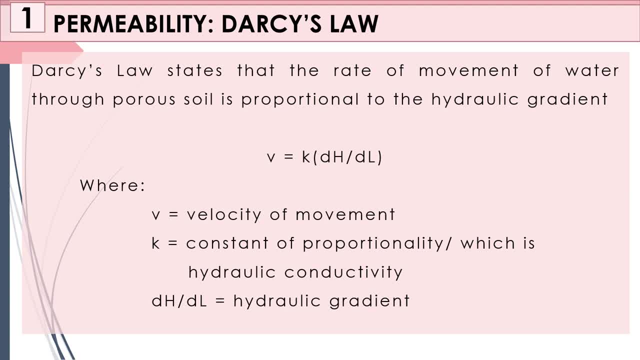 calculus. no, because you see DH over DL. So yung DH over DL na yan is nakuha no gamit yung mga pag-derive ng equation, So siguro hindi na tayo mag-derive, Okay. 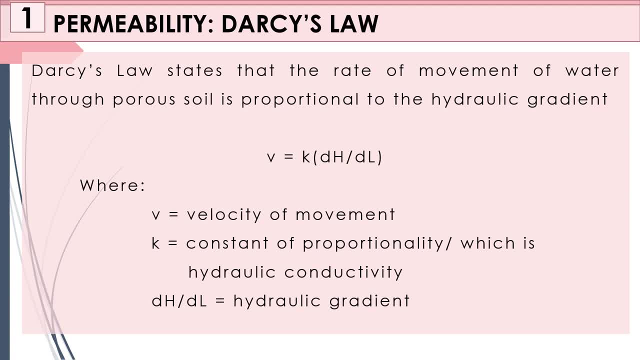 But then again, DH over DL. no, is tinatawag yung hydraulic gradient And normally on the other book, no DH over DL. okay, that is in a variable of. I Sige lang. ididiscuss natin yan. 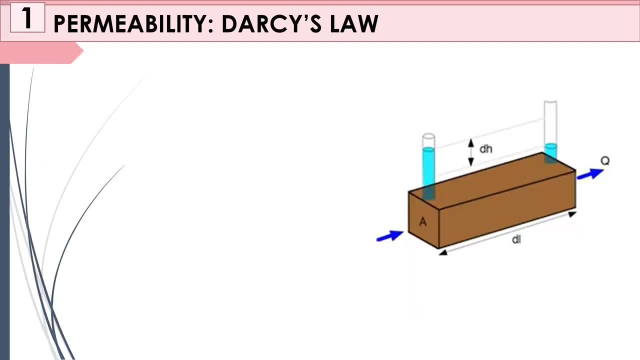 Okay, So this is the example of your permeability. So you have here your piezometer, which is, kukunin natin yung difference between the piezometer one and your piezometer two. So, DH dyan, is the difference between: 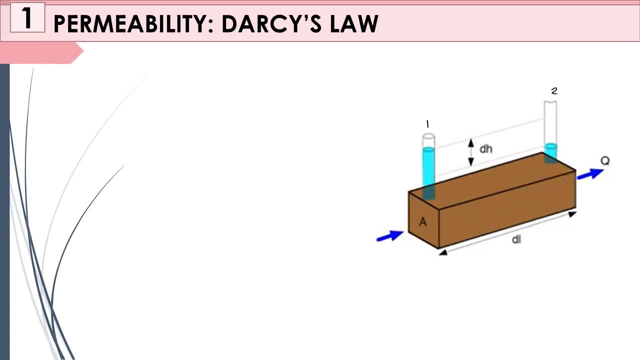 the height of your piezometer one and piezometer two. Okay, So as I've said earlier that yung permeability natin is in laminar condition, So in order for us to get the value of your H, okay, 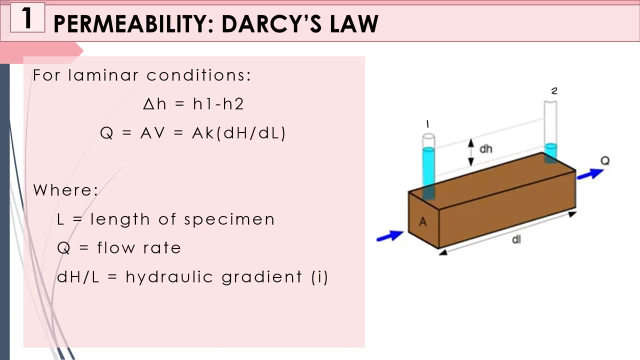 the value of your H. that is the difference between H1 and H2, where ito yung ating H1., Ito naman yung ating H2.. Okay, So Q is equals to AV Yan, yung nakilala natin during. 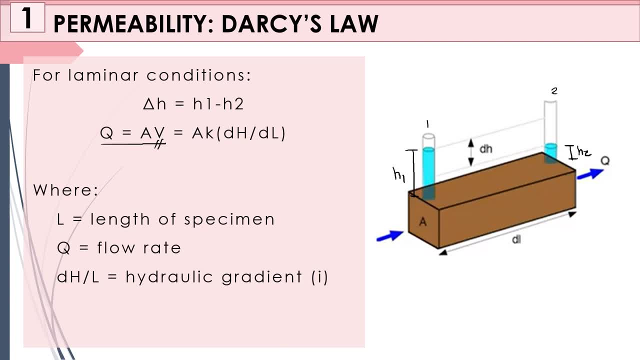 the hydraulics. But dito sa ating permeability, okay, tatawagin natin yung Q natin as A-K-I, No, Or Aki, Or dati. we did memorize this one as. 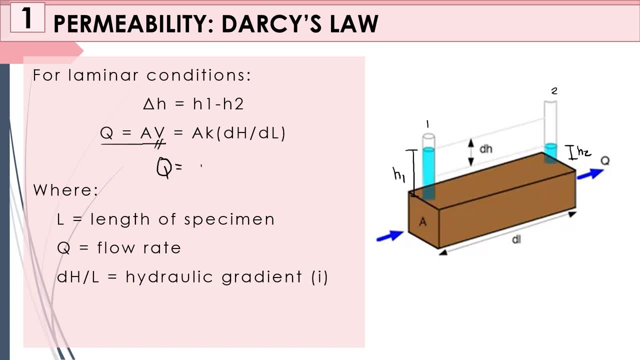 Kia. no, Where Q is equals to K-I-A Kia. Okay, Where your K is your hydraulic conductivity, or your coefficient of permeability, and your I is your hydraulic gradient, That is DH over DL And you have your A there that. 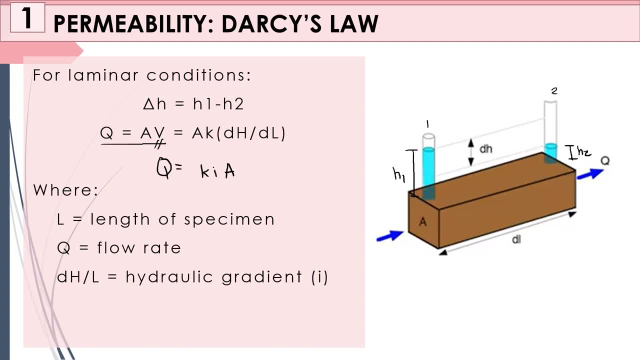 would be the area. Okay, But I want to emphasize yung area na pinag-uusapan natin dito. Okay, Yes, that is the cross-section area, But take note, no Kung alalang nyo doon. 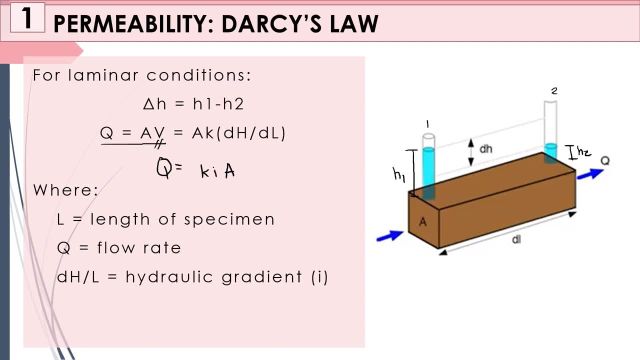 sa definition, kanina, that yung area na pinag-uusapan nito, natin dito, is the area perpendicular to the flow. Okay, So sabihin natin ito: yung soil solids natin, or 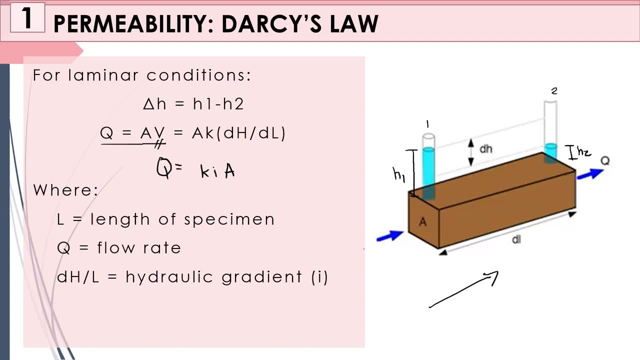 yung soil ninyo, and then ito yung flow, Yan, yung flow na force. Okay, Yung pinag-uusapan natin is the area perpendicular to the flow. So if this is the flow, this is the. 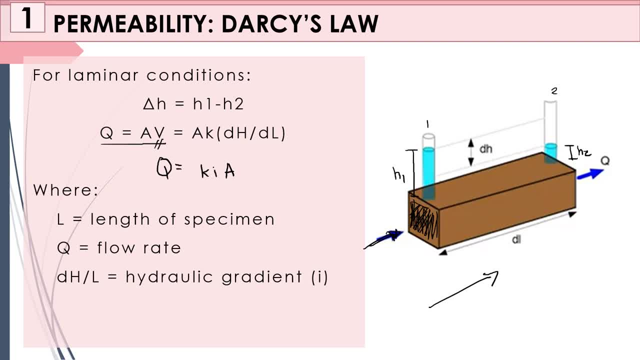 area. Okay, So that is perpendicular. Kita nyo naman na no Yan highlight na lang natin Yan perpendicular to the flow. Ito yung area na pinag-uusapan natin, Okay, And 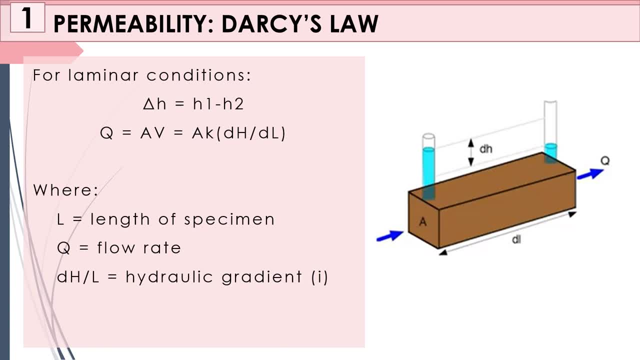 ano pa bang pag-uusapan natin dito? L, that is the length of the specimen. So saan naman natin makikita yung length dito If the area is perpendicular to the flow? ang length naman natin dito. 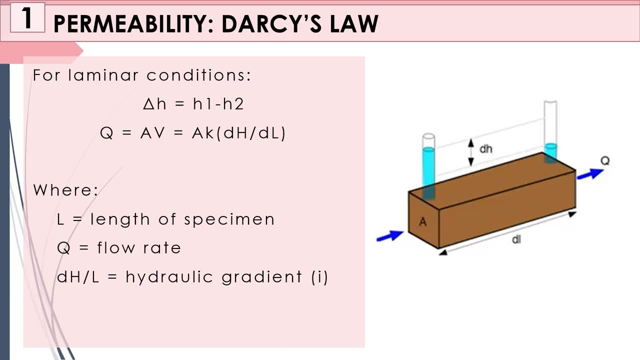 is, it must be parallel to the flow. So if you have a flow like this, ibig sabihin yung length natin is parallel to the flow. Again, area is perpendicular- to ano ba ito- To the flow. 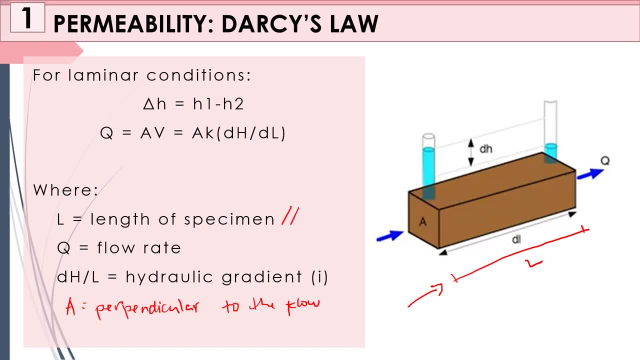 While your length is ganito na lang, parallel Di ba, Parallel sil mo yan to the flow. So therefore, your Q or your flow rate, that is, kia or K-I times A, where your- I is the difference. 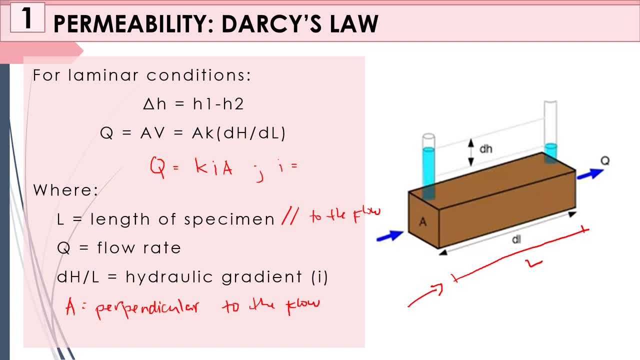 between your H1 and H2, or that would be delta H over L, because that is dH over dl. Ito Yan, eh Okay, Actually dinerive talaga yung formula na yan. pero hindi na lang natin ito. 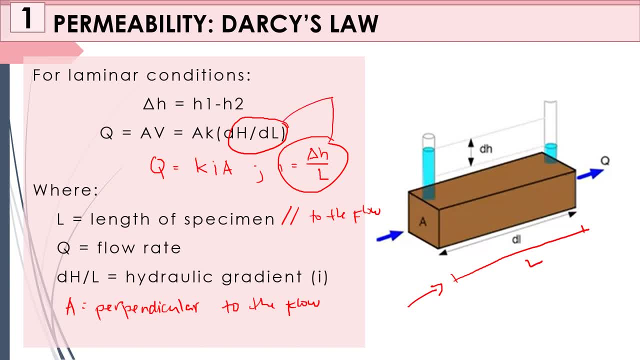 ididerive, kasi sobrang taas na. But you can look for the book of Braja M Das Maganda, yung book niya because it is well explained, yung on how the hydraulic gradient is derived- Again Braja M. 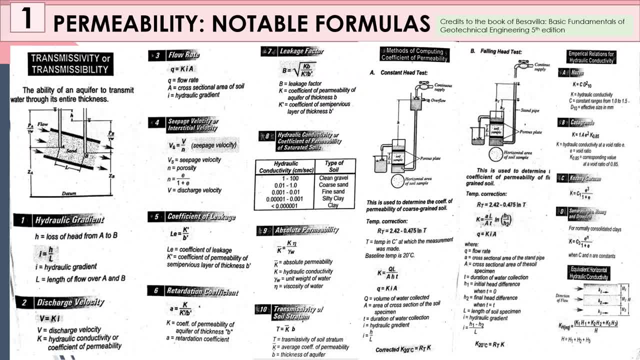 Das Maganda, yung book niya. Okay So, yun ah. So for this topic dito sa ating geotechnical, which is matik naman na we will deal with lots of formula, Okay So. 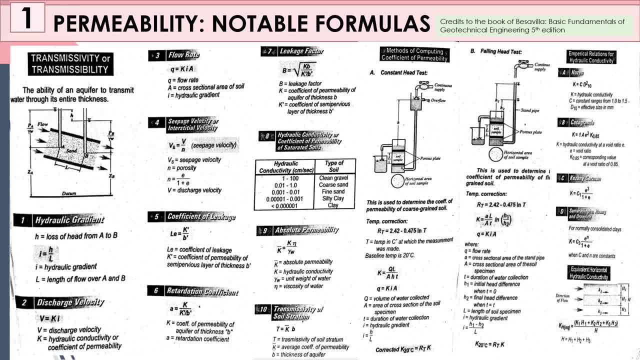 ang daming formula sa geotechnical engineering. So that is why you need to practice yourself in solving more problems, because kapag lagi natin sinusulat yung formula, na-memorize natin siya agad, Minsan nga, kahit hindi natin iniisip. 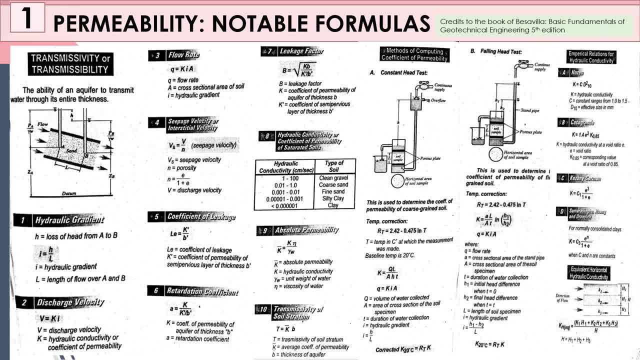 nagsusulat tayo, yung kamay na natin mismo yung nagsusulat agad sa formula, Kasi memorize na nung kamay natin. Buti pa yung kamay natin memorize yung formula. 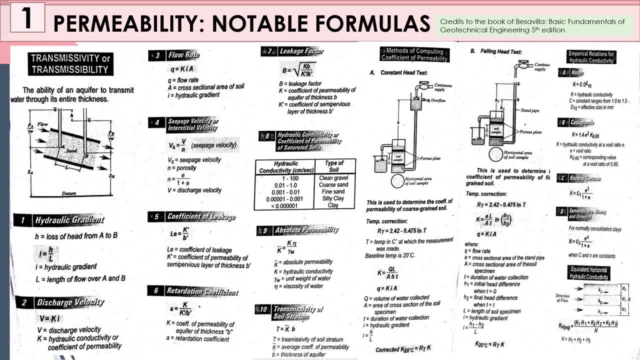 But then you know that is very true na kapag sulat ka nang sulat or solve ka nang solve ng problem, sulat ka nang sulat ng formula na may memorize mo na agad Without you knowing na sinusulat mo na agad. 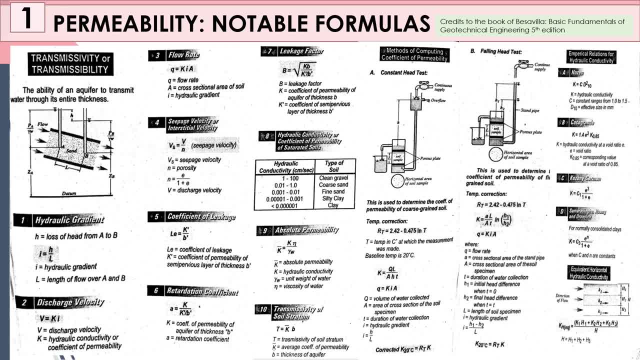 yung formula, without you knowing, na memorize mo, na pala siya. Okay. So these formulas, I took it from the book of Besavilla for the Basic Fundamentals of Geotechnical Engineering, 5th edition. 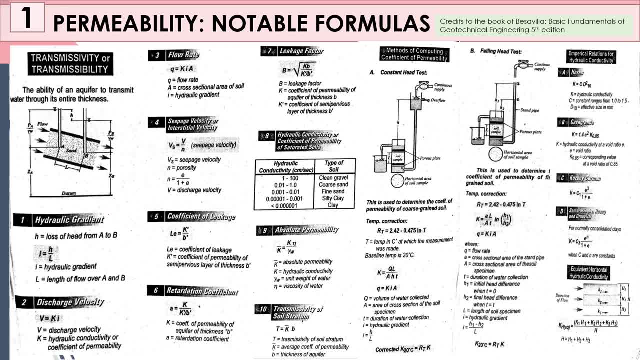 Okay, So you have here your hydraulic gradient, which is yung napag-usapan natin kanina. That is, I is equal to H over L, But H here is the difference between your H1 and H2.. Ito yung A natin, This is. 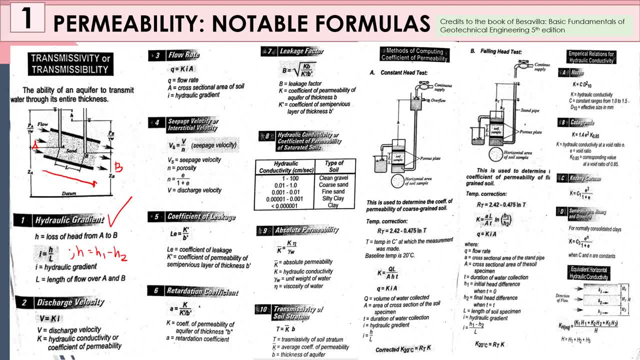 the A and this is the B, So ito yung flow ng fluid natin. So gusto ko lang ibahin yung concept ninyo na kung nasaan yung mataas na part, pwede natin isipin na doon ang galing yung. 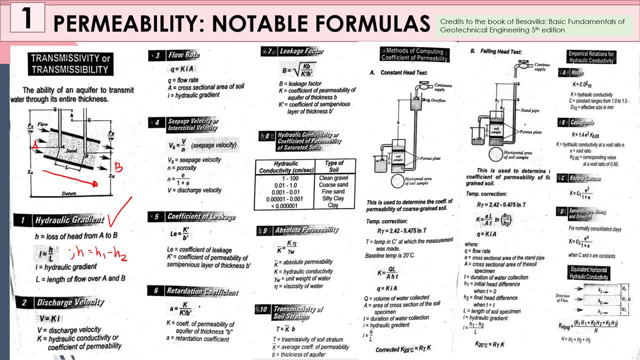 fluid, no Pababa. So take note, pwede din magkaroon na galing sa baba papunta sa taas yung fluid. Next is you have your discharge velocity. Now you can have the formula of that as K times. 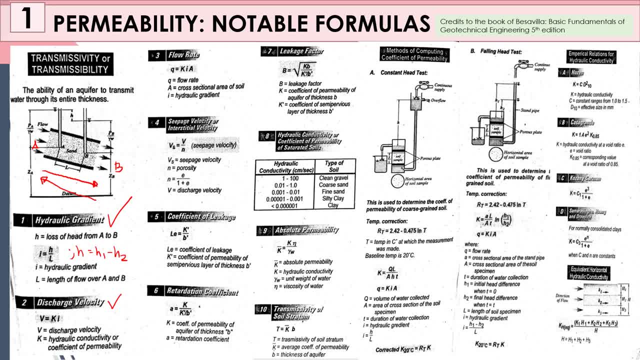 I Okay Again, where your K is your coefficient of permeability. So you have here your flow rate. small letter: Q na lang, siguro yung ginamit dito na Besavilla, para hindi malito, no, Sa Q is equal. 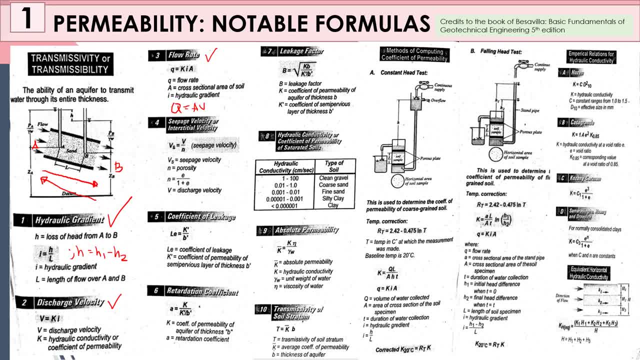 to AV, But that is the same, which is talking about the flow rate. Okay, So you have here your seepage velocity, or tinatawag din siyang interstitial velocity. Okay, That is the formula. of VS is equal to V over. 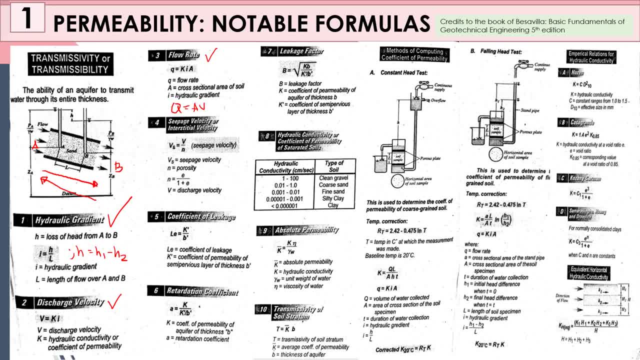 N where your N? that is your porosity. And take note, yung V natin dito is your discharge velocity. Okay, And we have another miscellaneous formulas. Okay, Kayo na lang tingin yan. So we have here a table. 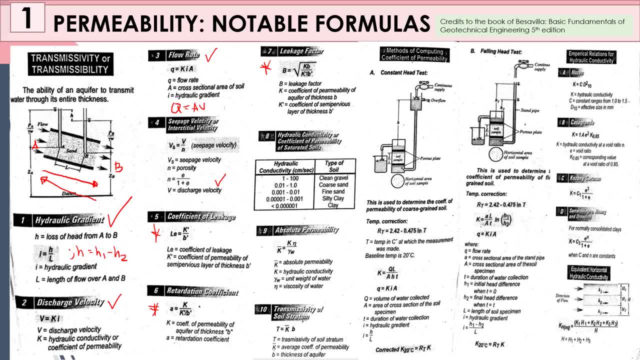 for your hydraulic conductivity for a saturated soil. So hydraulic conductivity that is in a unit of centimeters per second. So you have 1 to 100. type of soil is clean and clean gravel 0.01 to 1, that is. 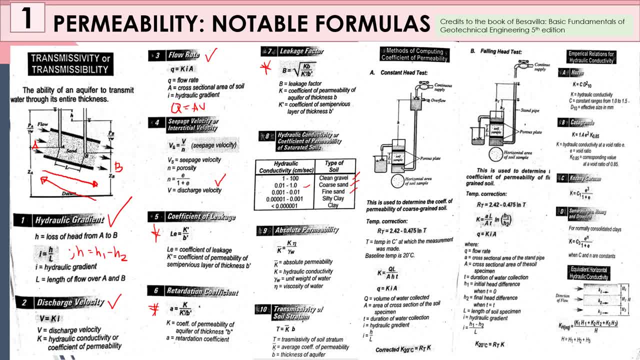 coarse sand. Next is you have for your fine sand stilted clay and clay. Okay, Normally yung lumalabas talaga ng formulas dito is halos lahat ng to, But technically ito number 9 and number. 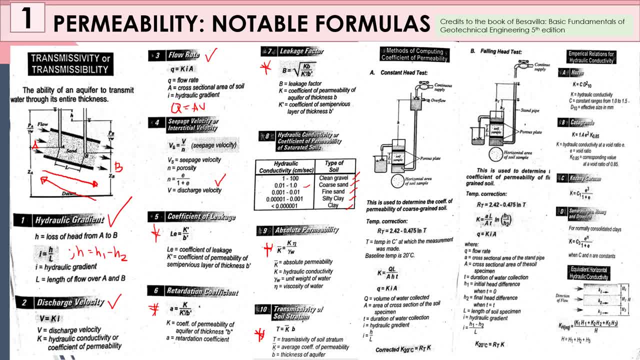 10. Yan, lumalabas talaga yan You have your absolute permeability and you have your transmissivity, transmissivity of soil stratum. Actually, itong number 10, lagi ko itong nababasa sa mga problems. 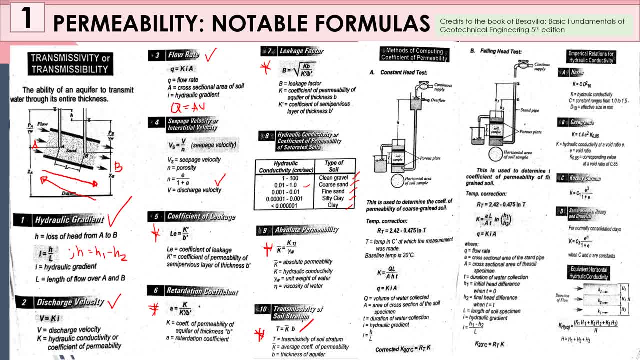 example. So, which is sobrang darilan ng formula, That is, T is equals to KB. So nakikita nyo, merong bar, yung K natin, or that is called K bar. No, Yung K bar natin, yan pinatawag natin. 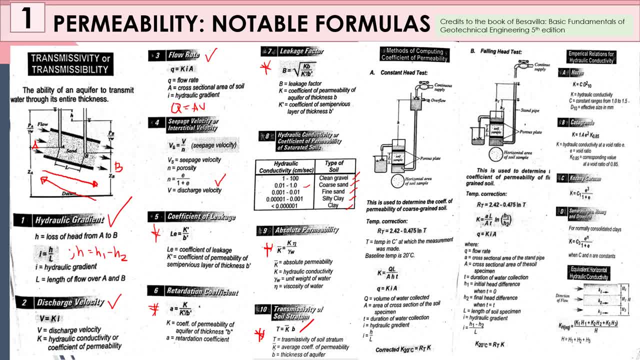 yung average coefficient of permeability. So K bar is not equal to K, Take note of that, Okay. K bar is not equal to K. Okay, So we have here additional formulas for our permeability. So meron tayo. 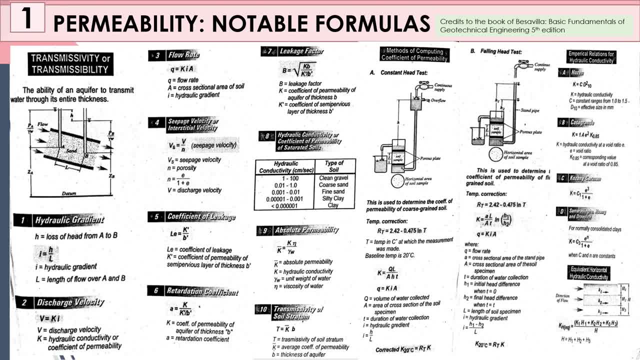 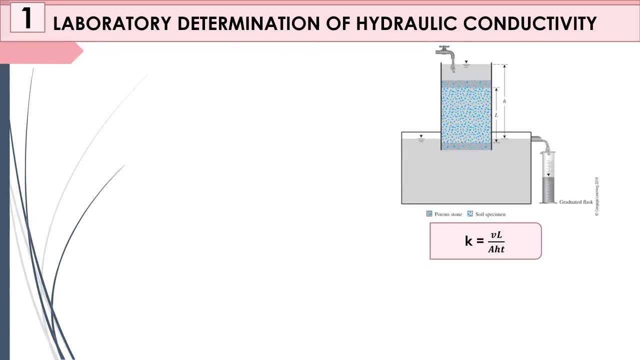 yung methods of computing: coefficient permeability. We have a constant head and we have a falling head, So empirical formulas meron din tayo dito. Okay, Sige. So let us talk about your laboratory determination for our hydraulic conductivity. 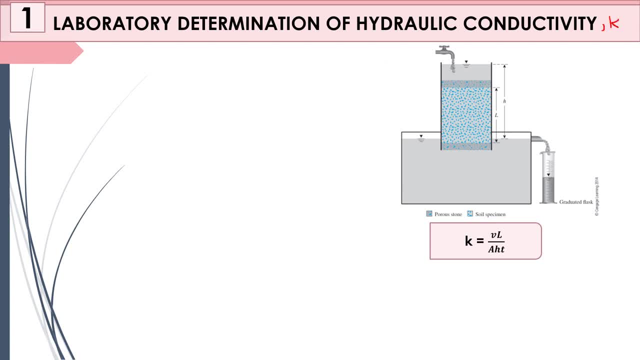 which is nga yung K natin. Okay, So this is our porous stone, Itong mga dots-dots na to Porous stone, yung tawag natin dyan, And then sa baba, okay, which is. 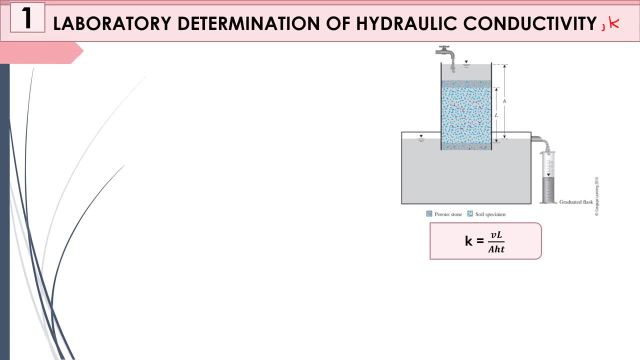 may gray na banda. that is your soil specimen, And we have here your graduated flask and dito naglalabas o nagdi-discharge yung ating fluid. So let us start with your constant head. So in this laboratory. 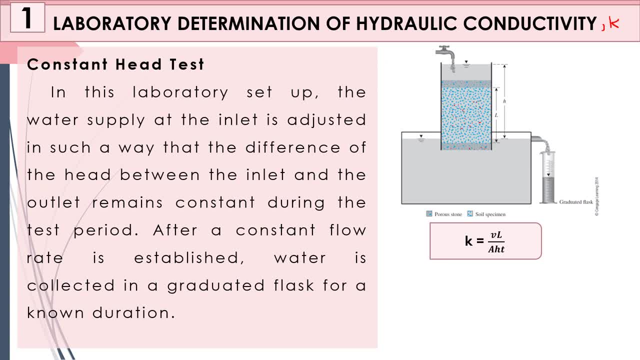 setup the water supply and the inlet is adjusted in such a way that the difference of the head between the inlet and the outlet remains constant. Okay, During the period or the test period. So, after a constant flow, the rate is established, The water is collected. 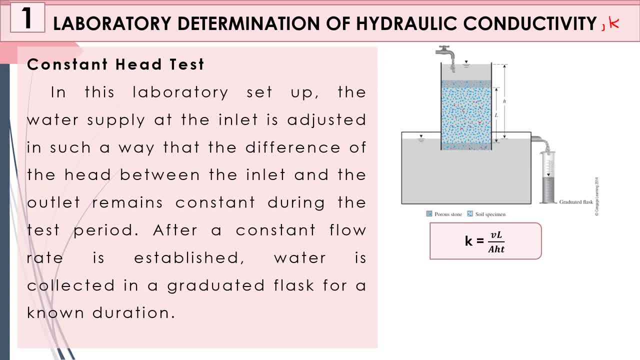 in a graduated flask for a duration known. So parang palang itong pareha sa tapik natin sa hydraulics, Which is yung constant head, Meron tayong rate of inflow, Meron din tayong. 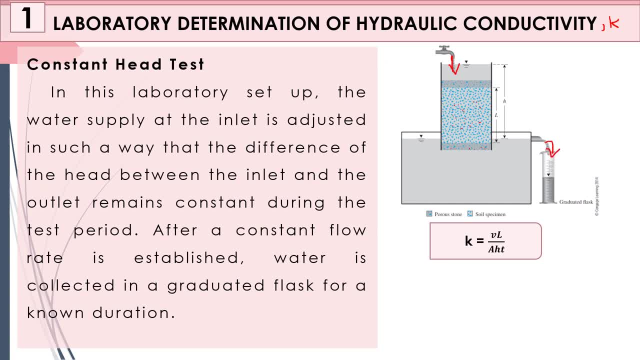 rate of outflow. Meron din tayong rate of outflow. So that is why hindi nagbabago yung ating head, Kahit na may nadidischarge palabas, Nadidischarge palabas ng ating 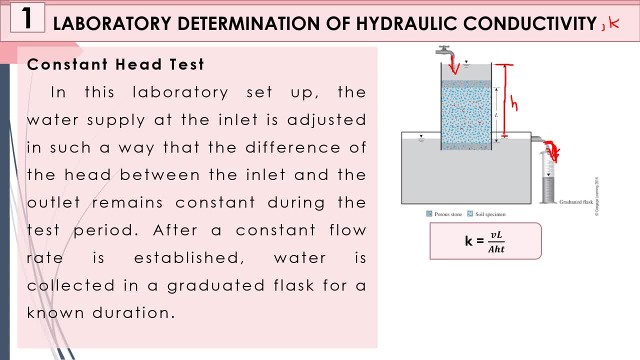 aparatus, So yung head natin doesn't change. So basically, kaya nga sya tinawag na constant head. So in order for us to get the value of our hydraulic conductivity, na that is in the formula of K is equals to VL. 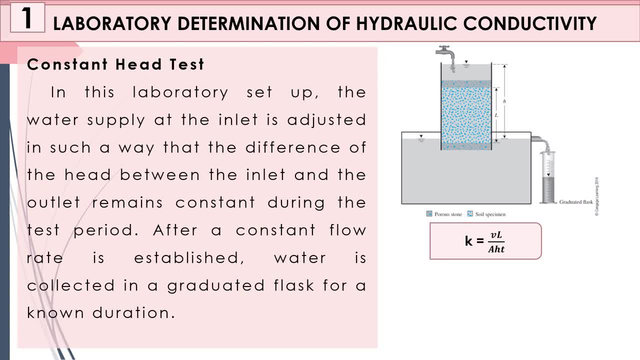 over AHT. Mom, bakit, kanina, doon sa mga formulas na pinakita mo, Sabi doon, kanina, that K is equals to QL over AHT. Actually, guys, that formula, this formula and this formula lang is the same. 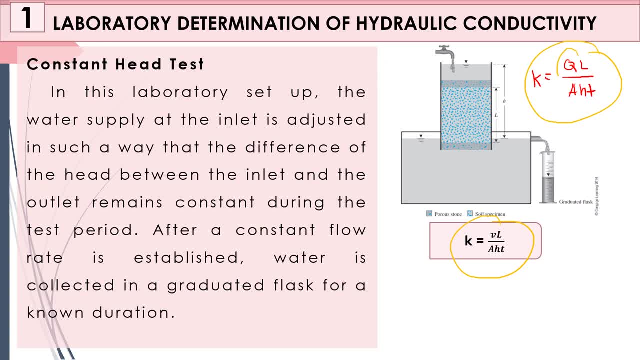 Okay, Dito kasi kay Besavilla: ginamit nya is Q, And then dito naman kay sa kinunan ko ng formula na to ginamit nya naman is V. I think, I think, I think no. 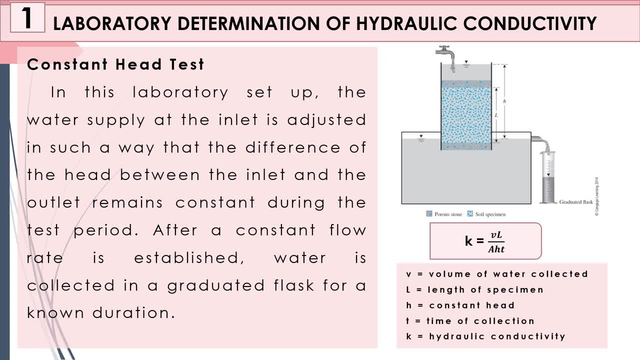 change nyo lang yung variable into V para hindi magkalito. Because Q there is not a flow rate. Okay, Yung minimin natin na Q dito sa formula na pinakita. ko kanina, no ibig sabihin ng Q. 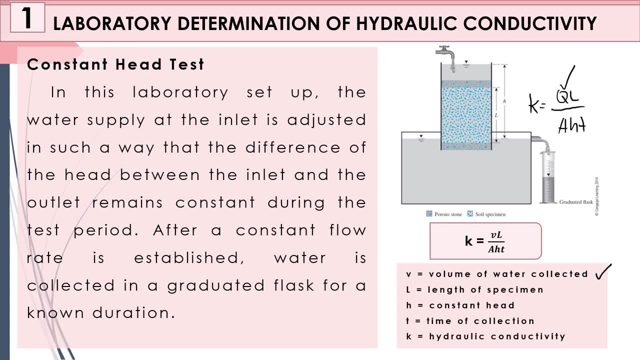 dito, that is the volume of water collected. Ibig sabihin volume yung pinag-uusapan natin. That is why dito inemphasize na V na lang, But regardless kung ito yung gagamitin ninyo, 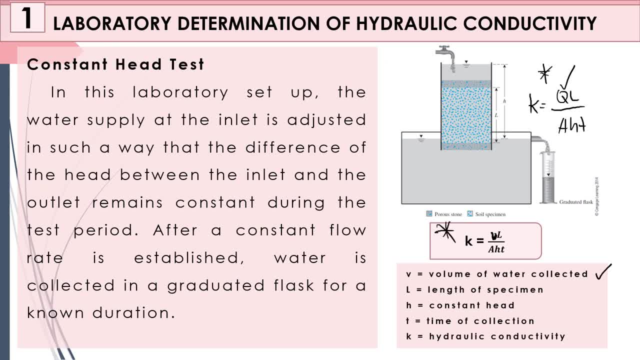 or ito parehas, lang naman yan yung lalabas. Okay, So L is the length of the specimen, H is the constant head, where T is the time of collection and K is your hydraulic conductivity. So during our 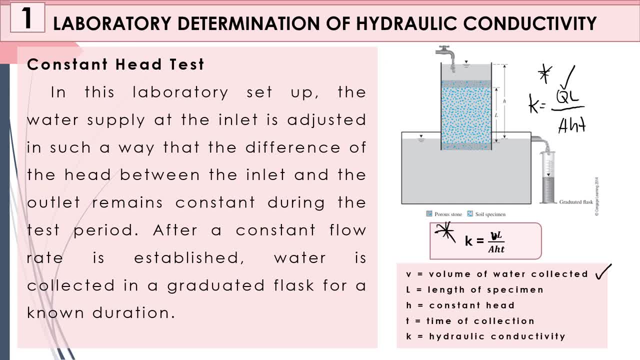 review. we have mnemonics for this, for this formula, So tinatama namin natin Bakit Q ito Ito rin kasi yung formula na mnemorize natin, Pero inalam lang namin yung definition. 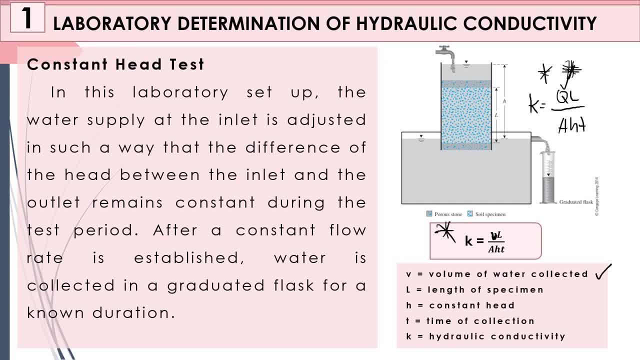 So Q L over A-H-T. So yung mnemonics namin dito is: kilat Or kidlat ba Kilat QL, This is your QL And this is your A-H-T. Kasi kapag itong formula na ito yung: 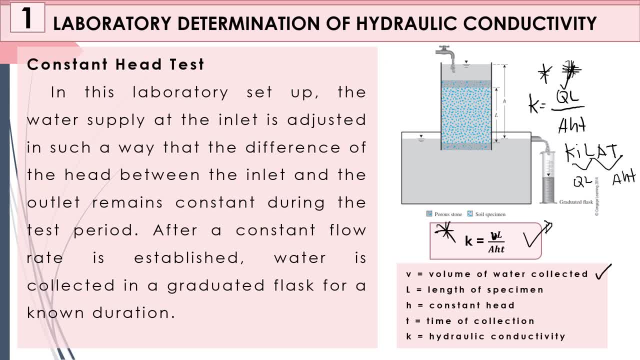 gawa natin ng mnemonics parang medyo pangit pakinggan, Kaya nalang balang mag-isip kung ano yun. So dito na lang, tayo sa kilat. Tandaan nyo lang that your Q. 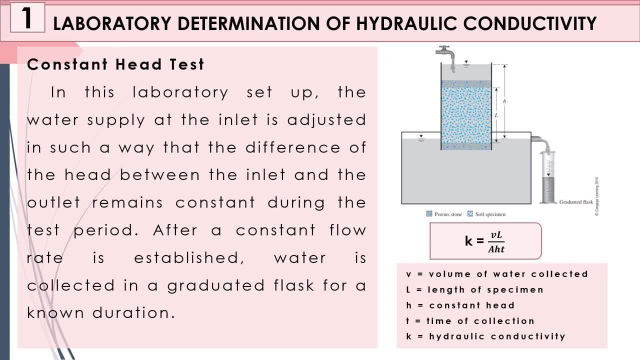 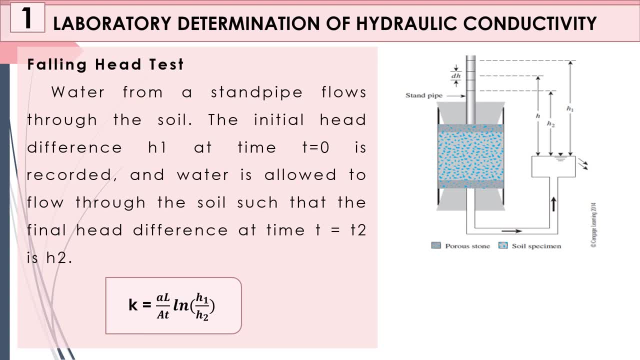 is the volume of water collected. Parehas lang naman yan. Another one is for the determination of your hydraulic conductivity. you have here your falling head test. Okay, So from a standpipe close to a soil, the initial head difference of H1. 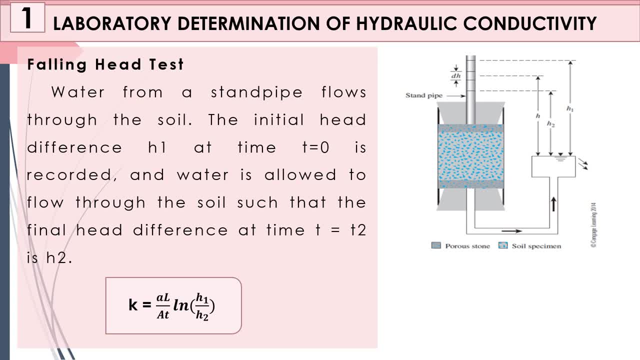 or your initial height, at time T is equals to zero And allowed, and the water is allowed to flow through the soil, such that the final head difference at time T is equals to T2, that is, H2.. So this is your apparatus, Okay. 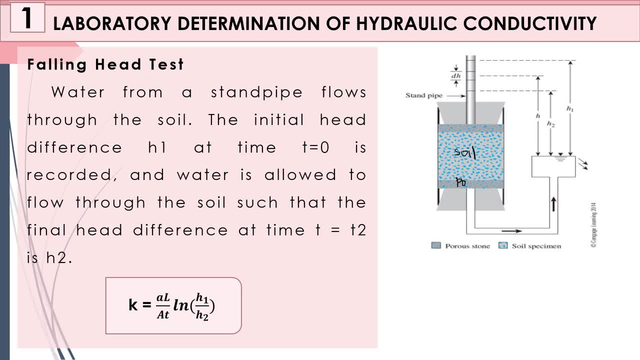 So this is your soil specimen and this is your porous stone. So sabi dito: meron tayong standpipe where nagpo-flow yung ating tubig, So dito nanggagalang yung tubig natin. 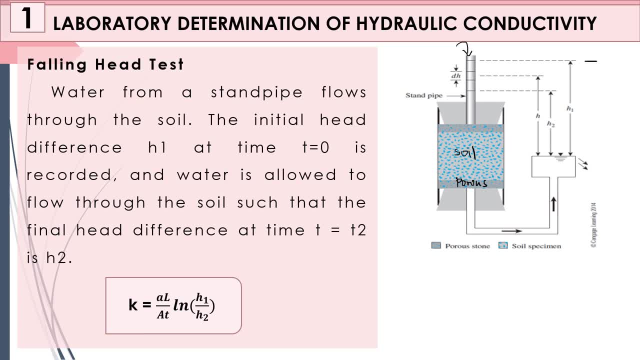 And then you have here your H1.. Okay, H1, natin yan Yung H1 ninyo, or your initial height, is nakukuha when time is equal to zero, Which makes sense. Ano nga siya Initial Pasimula pa lang. 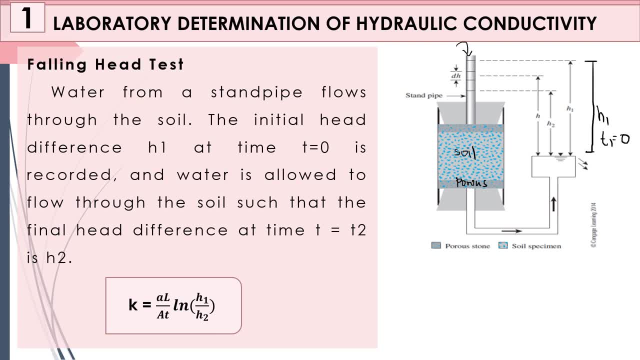 Therefore T is equals to zero. Therefore your H2 here, kukunin natin yung H2 natin- when T2 is equal to T And you have the formula for your falling head test, and that is K is equals to AL over AT. 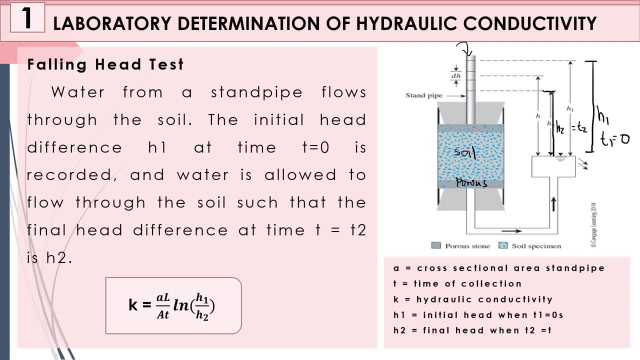 ln. H1 over H2.. Where your small letter A is the cross-sectional area of your standpipe. Ito Area nito, Okay, T is the time collection. K is your hydraulic conductivity, H1 is your initial head and H2 is. 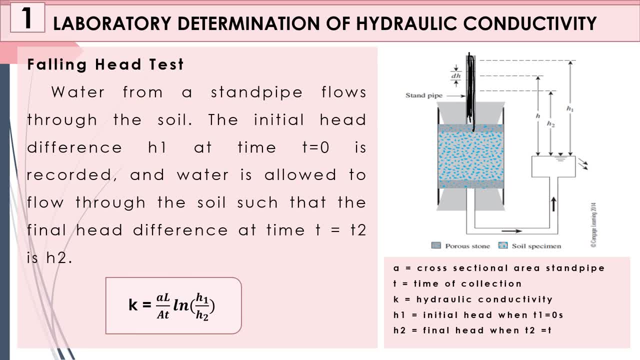 your final head. So dito share ko lang ulit yung pneumonics namin for this one. Kung babasahin natin ito, Ano ba yan Kalat. So kalat, kalat lang, ha, ha, ha. O yan yung aming pneumonics. 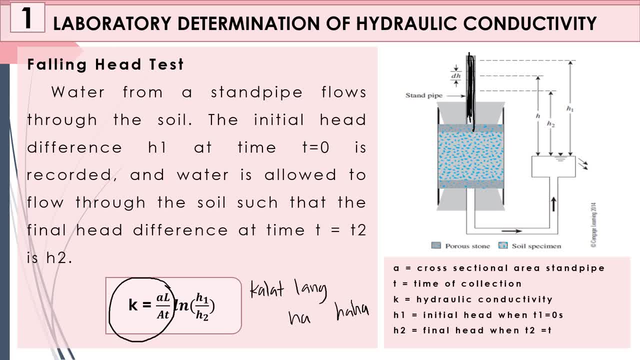 for your falling head test. Kalat lang, ha ha ha. O kayo na bahala. kung ayaw yun, ang pneumonics na ganyan, Kayo na lang gumawa. Okay, Basta that's how we memorize the formula. 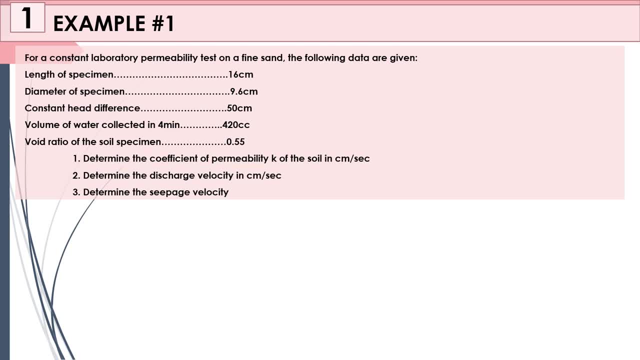 during. Okay, so let us try some example to better understand this topic. So we have here for a constant laboratory permeability test on a fine sign. The following data are given So: length of the specimen, diameter of the specimen, constant head difference, volume of water. 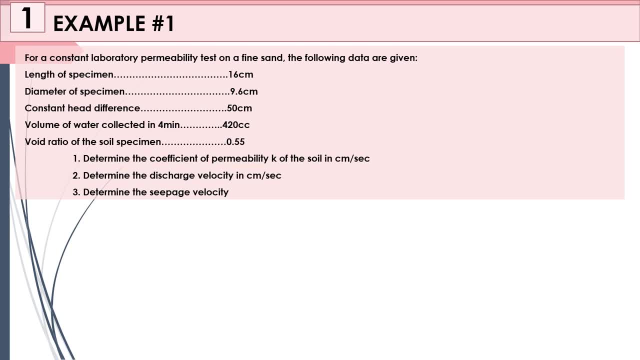 collected in 4 minutes, which is 420 cubic centimeter, and then volume of- I mean that is your void ratio of the soil specimen. So what is asked is for the value of our coefficient of permeability, that is your K Discharge velocity, that 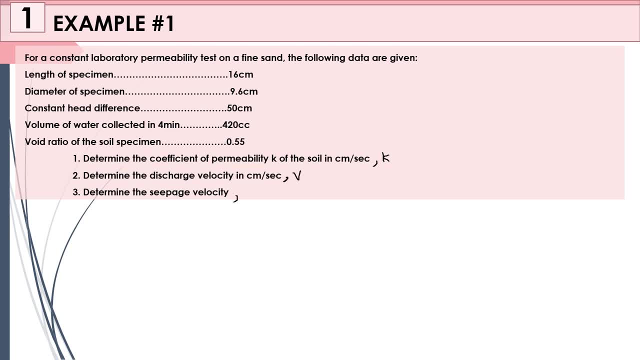 is your V and your seepage velocity that is your Vs. So what type of laboratory test is this that we are solving? Yes, that is correct, That is your constant laboratory permeability test or, basically, that is your constant head test. There is a constant. 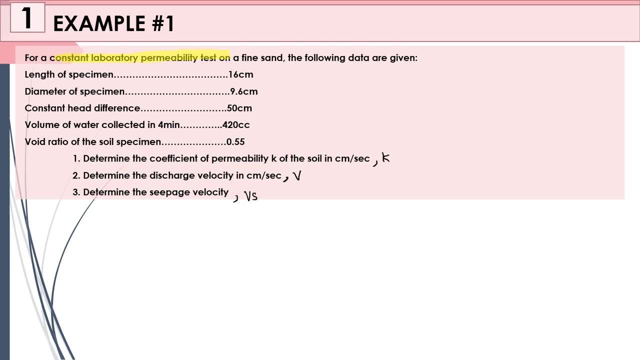 word that is a dimatic. So, going back, what is our formula for your constant head test? If you remember, that is your. that is, your K is equal to KILAT. Is that correct? KILAT? Again, where your Q is. 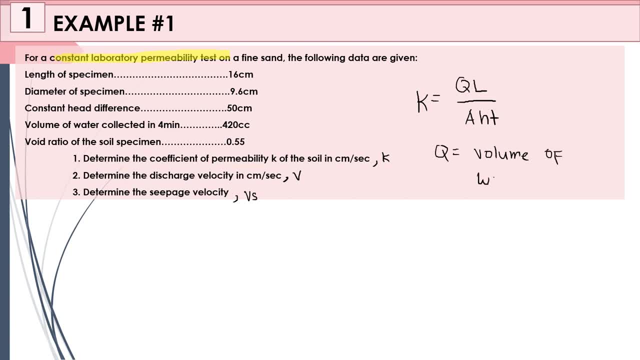 your volume of water collected. Take note of that. it is not rate of flow, But we can play with it so that we don't get confused. That is it. Let us just follow the formula that was given. So let us go to the solution. 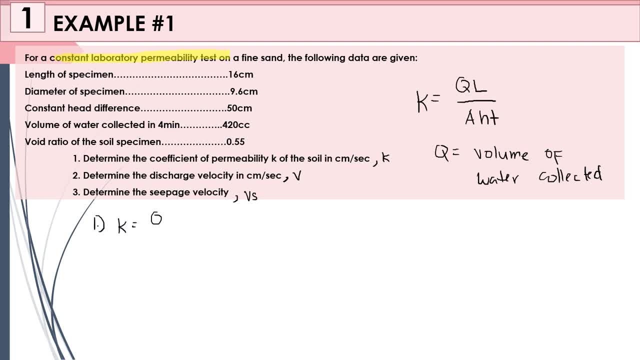 Let us find the K. K is equal to QL over AHT. K is equal to how much is our Q? That is 420 cubic centimeters. Next is your length. Your length is 16 centimeters over our area. What is our area? 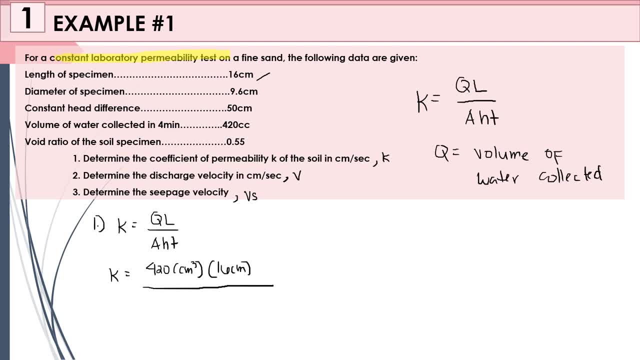 here The area is not given, But the diameter of our specimen. Therefore, that is Pi over 4 times 9.6 squared. Therefore this unit is centimeter squared also. Okay, Next is to multiply by the value of our H. What is our H here? 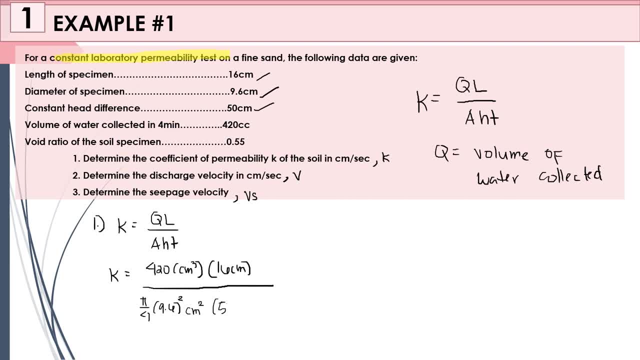 This is it? Constant head difference, which is 50 centimeters, And T is for the time collected. How much is that? That is 4 minutes. So what is the question here? The problem became strict. He said: let us find the. 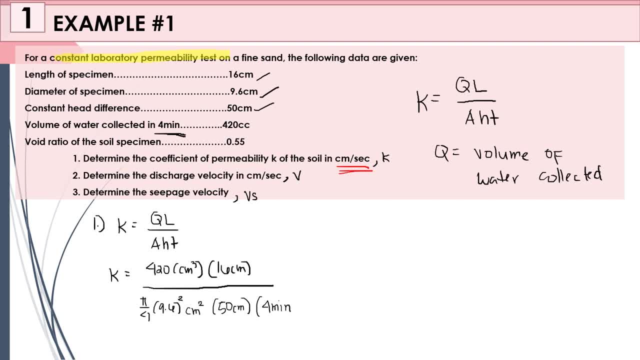 coefficient of permeability, But that should be in centimeter per second. So therefore we need to convert minutes to seconds, And we know that 1 minute is equivalent to how much? 60 seconds? Okay, So cancel the units so that we 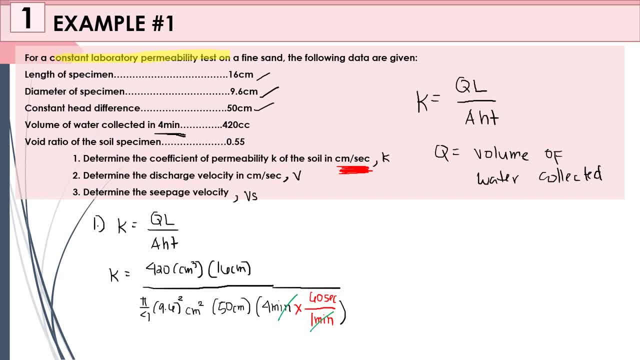 are not confused. So minutes here will be cancelled. Centimeters here will be cancelled. Centimeters squared and cubic centimeter are cancelled, But there is one left. Okay, Therefore our unit is centimeters and seconds. Okay, Using your calculator. 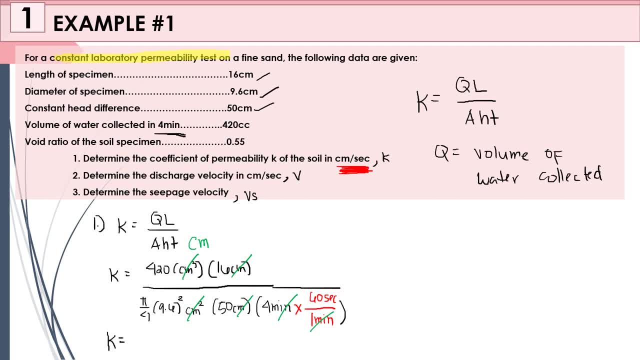 can you get the value of our coefficient of permeability? Okay, And can you check if the value is 0.078 and the unit should be in centimeter seconds? Let us check if the value is correct And that is the answer. 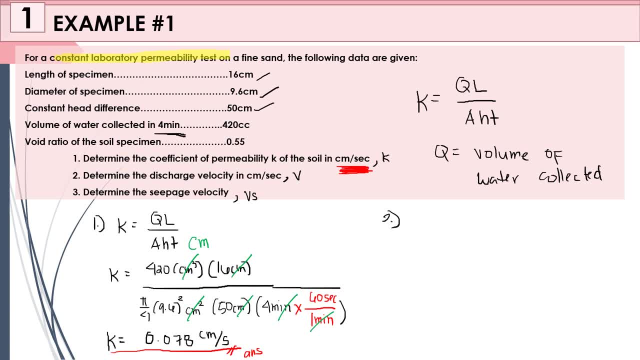 Okay, Let us go to number 2.. We are looking for velocity. Okay, So we are looking for velocity from discharge. So what is the formula of our discharge? Right, That is, Q is equal to Av. Where your Q here? what is our Q? 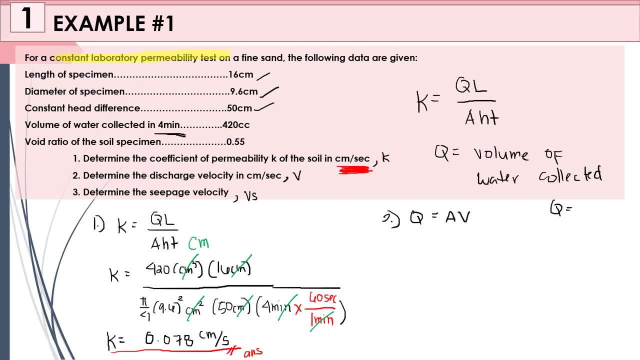 Right, Our Q should be in volume over time, Okay. Or that is in cubic centimeter, That is, in cubic meters per seconds, Or it can also be cubic centimeter per seconds. Okay, Let us erase it, So don't be confused. 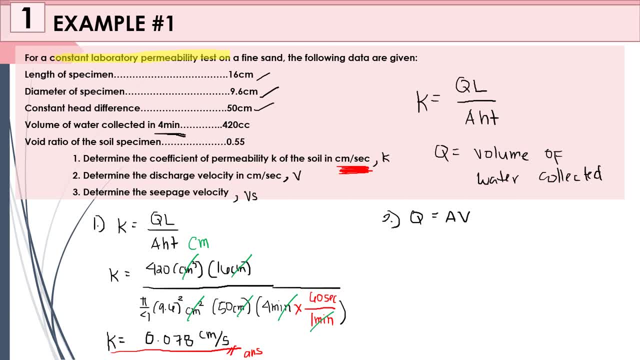 Because here in our formula, in coefficient of permeability, our Q here is volume of water collected. Number 2, we are asking here is the discharge velocity. So where can we see our discharge? I mean discharge velocity, Right In flow rate. 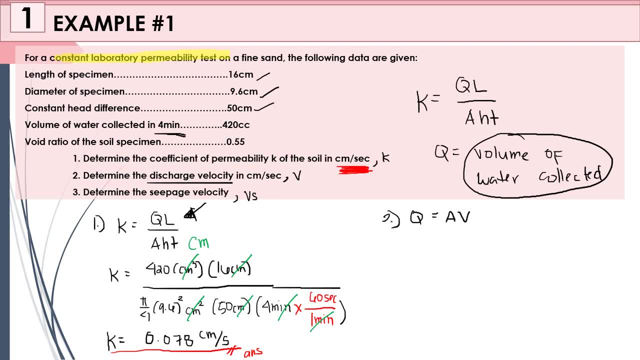 So I will use this Q Right, So don't be confused. Okay, So for our Q that would be 420 cubic centimeter. over the time that it took, That is 4 minutes. It is equal to the area. 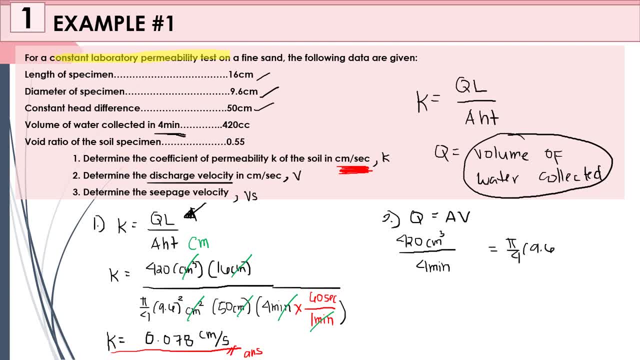 which is pi over 4 times 9.6 squared. So I will put here centimeter squared times V. Okay, So it became strictly the same problem. It says discharge velocity in centimeter per seconds. It means: let us convert it again. 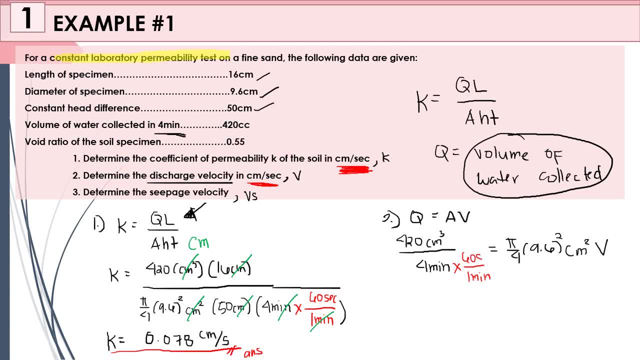 to seconds. One minute is 60 seconds. Let us cancel the unit. Minutes here will be cancelled. Okay, Centimeter squared cubic centimeter. cancelled will leave one. Therefore, the unit we left is centimeters and seconds. So kindly solve for the value of. 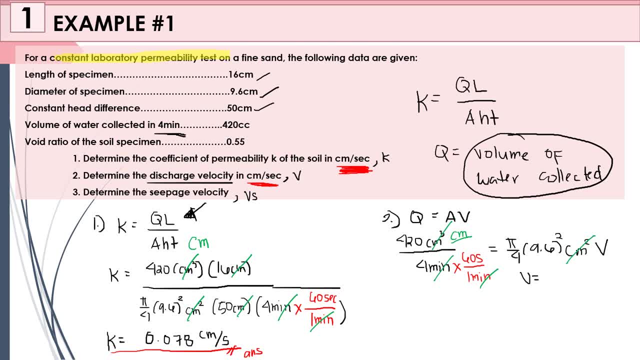 our V And kindly check if the value is 0.024 centimeters per seconds. And that is answer number 2.. Okay, So let us start number 3.. So it says in number 3, the seepage: 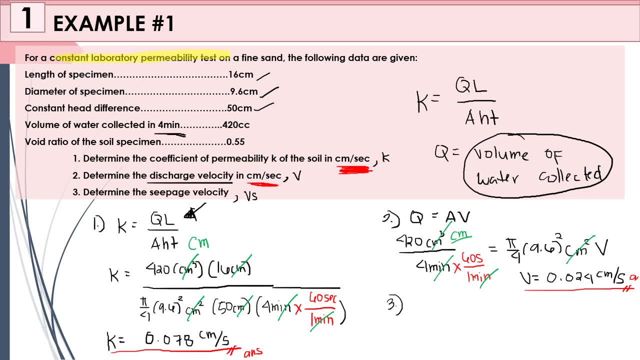 velocity. So it is not a strict unit, So it is a matik unit. The unit we will use is centimeter per seconds, But what is the formula for our seepage velocity? So, going back to the formulas that I showed earlier, 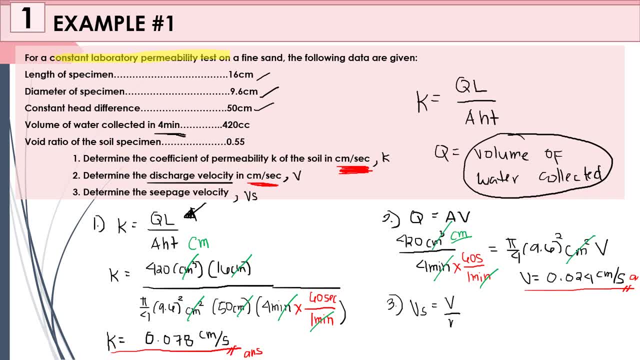 the formula is: Vs is equals to V over N, So we already have V, where there is a unit of centimeters per seconds. That is why I assumed that our unit is centimeters per second, So Vs is 24 centimeters per second. 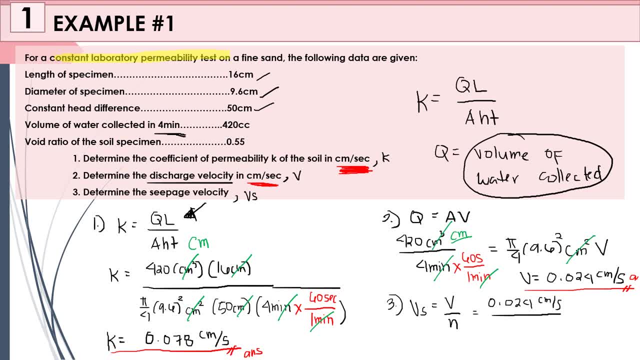 divided by the porosity. Did we provide any porosity? No, we did not. So what is the porosity that we provided? What is the porosity that is provided? We provided the void ratio, So we all know that we can obtain. 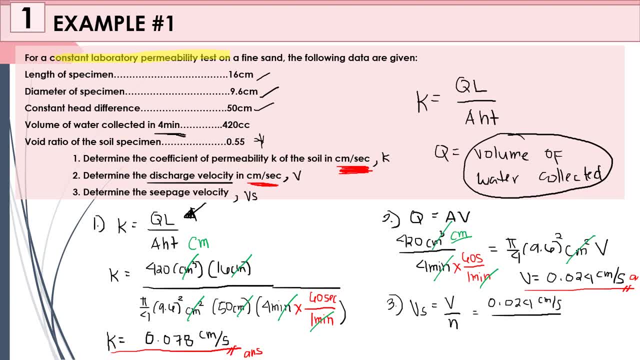 the porosity if your void ratio is given. So what is our formula for porosity? 1 plus e. so therefore, that is 0.55 over 1 plus 0.55. ilan yan, that is 0.355. okay, lagay na natin sya sa equation: 0.355. so. 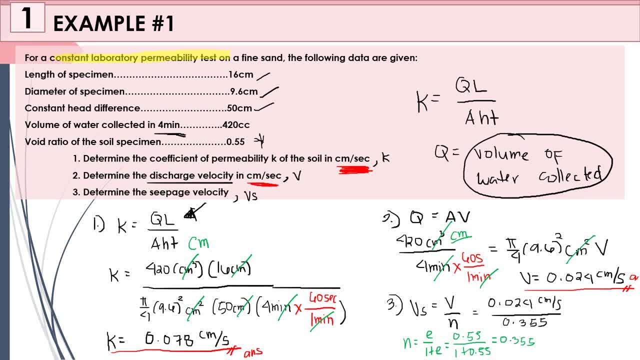 0.024 divided by 0.355, and that is equal to how much pakicheck if the value is equivalent to 0.068 centimeters per second? and that is our answer for that problem. okay, so let us proceed to example number two, which is: 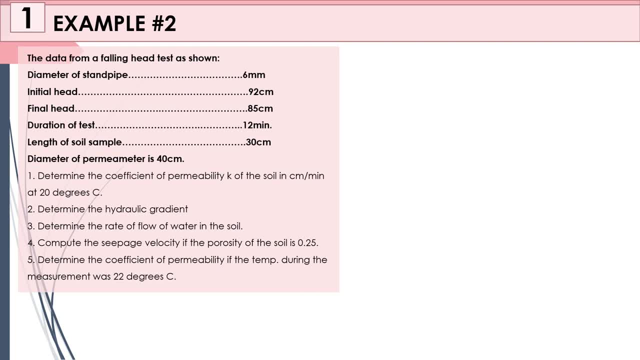 0.024 divided by 0.355, and that is equal to how much for the falling head na naman. so example number two states that we have a data from a falling head test, as shown. so we have a diameter for your standpipe, initial head, final head, duration of 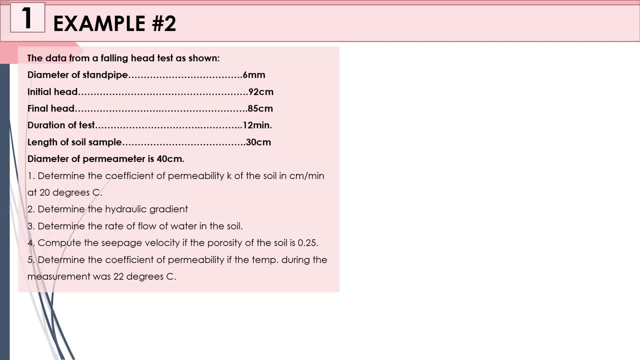 the test length of the sample and the diameter of your permeameter or your soil. no, is 40 centimeters, so what is asked is for the coefficient of permeability, or your k in centimeter per minute. so again, the emphasize: 20 degrees Celsius. where now going back? 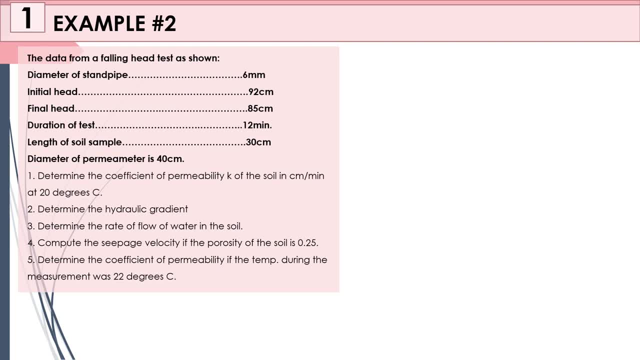 ancyphile. in express naman ant detail: Betterion K, not an hour, 20 degrees Celsius. next is your hydraulic gradient of hydraulic gradient, not attend. that is your I. next is determine the rate of flow in the water soil. rate of flowinking, that is your Q number for compute the seepage velocity. if the porosity between member 4 kms per minute, the evaluate the flow rate of flow. rate of flow in the water soil. 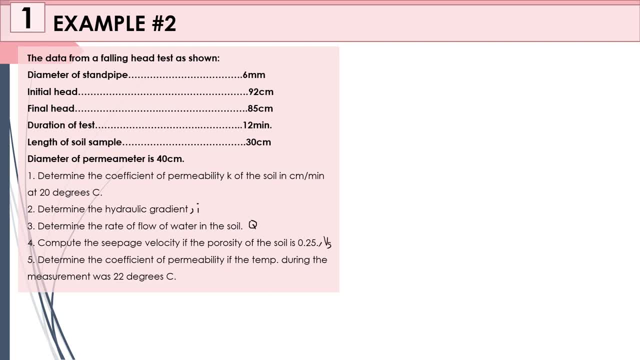 is 0.25. so therefore that is vs. next, number five determine the coefficient of permeability if the temperature during the measurement, or ito na, is 22 degrees celsius. diba sabi natin kanina, no sa ating principle that k is expressed in 22 degrees celsius, because your hydraulic 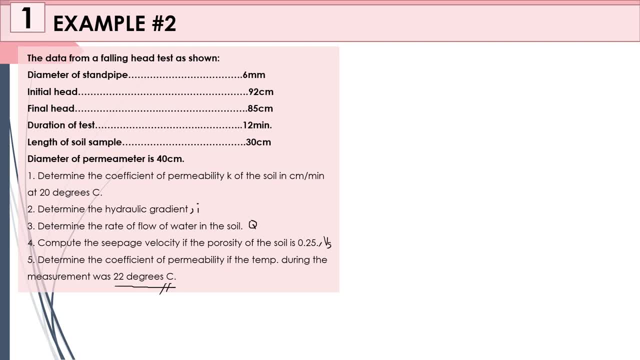 conductivity changes when temperature also changes. so ngayon, no, binigyan tayo ng 22 degrees celsius, ibig sabihin, yung k natin dito is not equal to the k na nakuha natin sa number one. okay, so simulan muna natin to sa pag solve natin sa first problem, which is your k. no, naging strict. 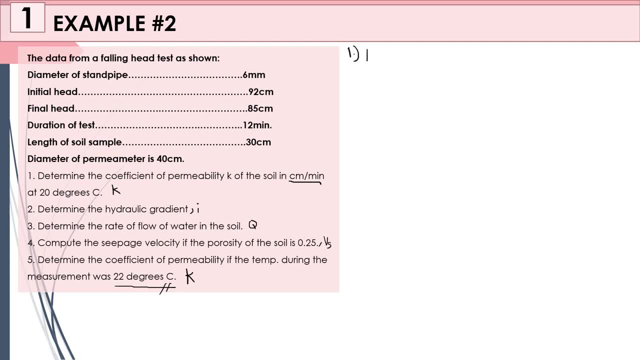 ang problem. that should be in centimeter per minute. okay, ano nga yung formula natin for falling head. that is your kalat long ha ha ha sana yung sulat ko, okay. so meron tayong diameter, puro diameter lang. wala tayong area. therefore, isa, solve muna natin. 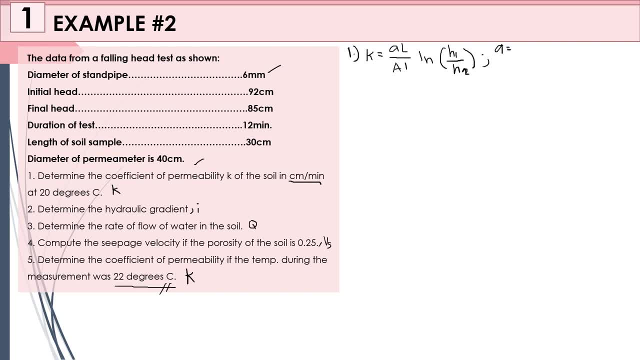 okay, small letter a is the area for your standpipe. so that is pi over 4 times 6 squared. ilan ba yan? oh, one ting naka mm pala to, so di lang sya. basta, basta six, okay. so ibig sabihin, balik tayo dito sa conversion. okay, be careful. oh naka mm sya, so lahat na ito is naka cm, so convert, wala tayong na gawa ico. convert natin yung mm to cm where iti divide lang natin to ng ten. 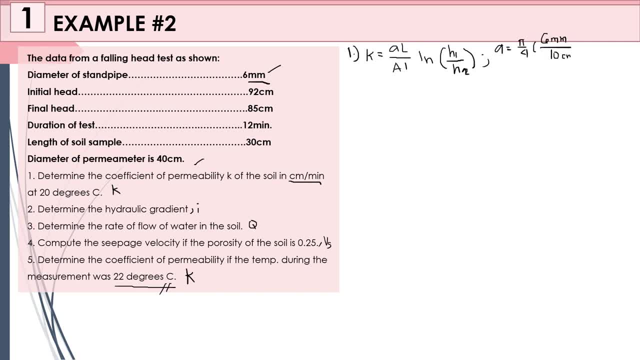 okay para maging cm, tapos square natin. So ilan ba yan, That is 0.283 cm2.. Be careful ha sa units. How about the area for our soil specimen? So that is pi over 4.. O ito hindi na natin i-convert, kasi binigay na agad siya in centimeters. 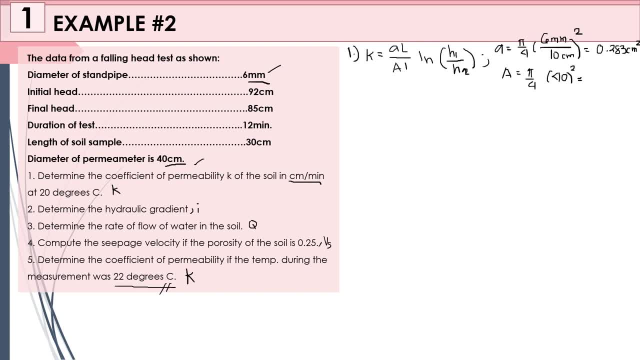 So you have 40 squared And that is 1,256.637 cm2.. Okay, and I think pwede na natin kunin yung ating coefficient of permeability for number 1.. And that is 0.283 cm2 multiplied by our L. 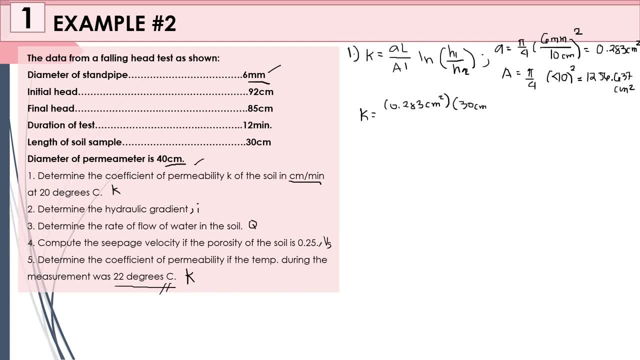 Ano ba yung L natin. Ah yun 30 cm Over, Over the area of your soil specimen. That is 1,256.637 cm2 times yung time natin, which is 12 minutes. So 12 minutes. 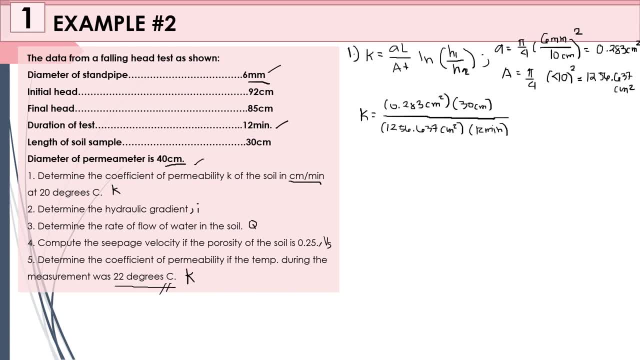 So no need to convert, kasi in minutes. naman yung ating hinahanap Ln of H1, initial head 92.. 92 cm over H2, which is your final Final head, 85.. Okay, siya, tinatawag na falling head, kasi from initial height to final height nagbabago. 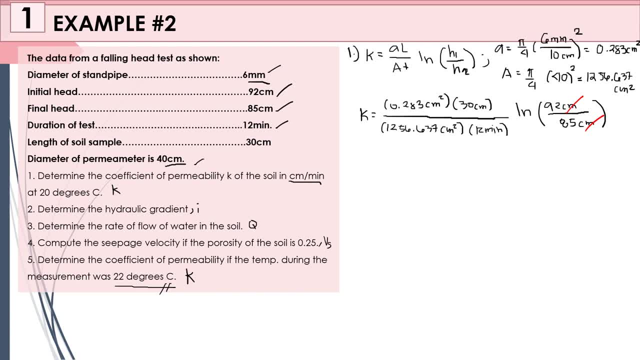 No, So centimeters here will be cancelled, Centimeters squared- cancelled. So ang magiiwan is centimeter per minute, which is pasok sa hinahanap ng problem. So ilan ba yung value ng K? Okay? 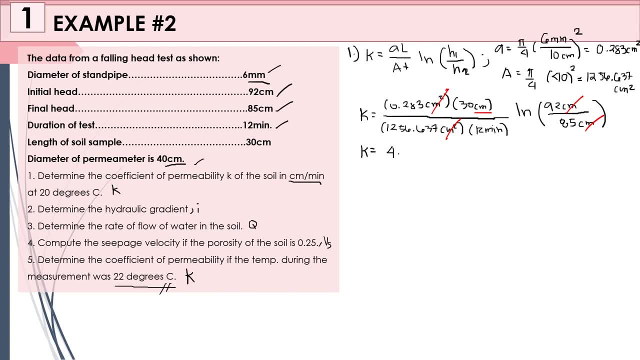 Okay, Kindly check na lang. if that is 4.456 times 10 raised to negative 5.. That is in a unit of centimeter per minute. Always nyong tatandaan yung unit kapag nagsusulat kayo ng final answer. 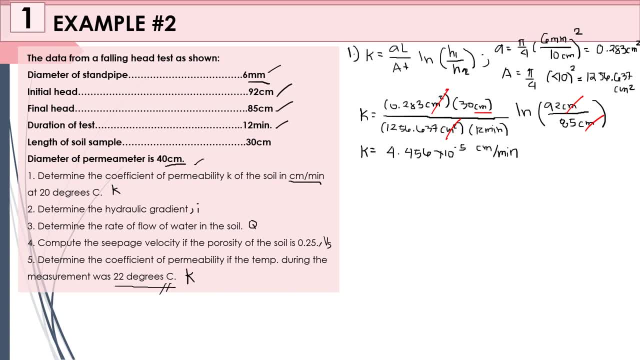 Kasi sayang hindi makikredit yung answer ninyo. kapag walang unit, Yan No, inulit, patikwi rin naman. Okay, Number 2,, hanapin natin yung hydraulic gradient ninyo, which is your variable. I. 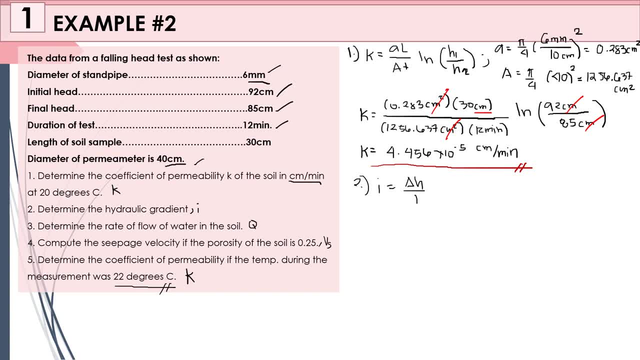 And that is the formula of delta H over L, Or that is the difference between H1 minus H2 over L. So therefore that is just 92 minus 85.. So anong unit itong dalawa Diba Centimeter? 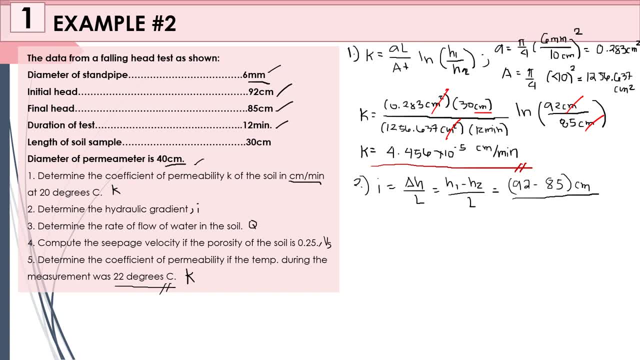 Centimeter Divided by L, which is 30. And that is also centimeter. O tingnan nyo to Units here will be Cancelled. Ibig sabihin your hydraulic gradient is unit less. So ilan yung I natin. 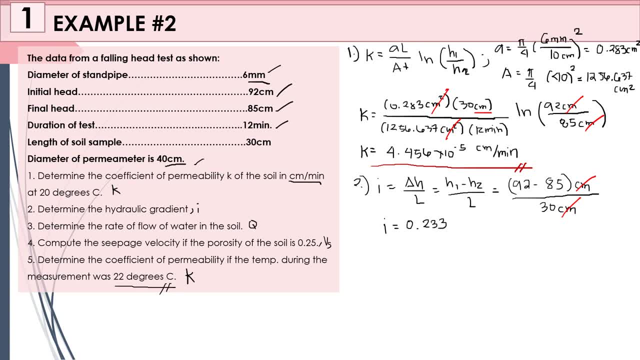 That is 0.233.. Pakicheck na lang yung value. Okay, Proceed tayo number 3.. Now determine the rate of flow, or your Q. Okay, So that is. your Q is equals to AV. Pwede ba natin itong magamit. 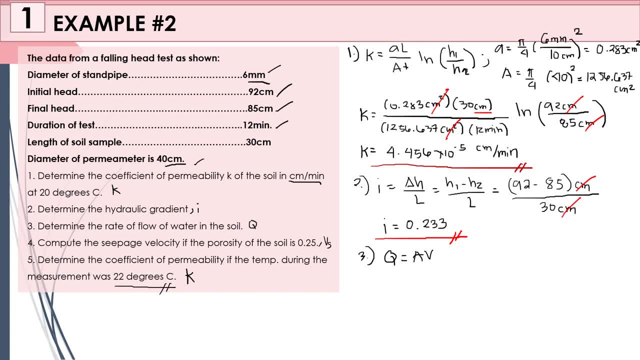 Hindi, Kasi hindi natin alam kung ilan yung velocity. No, Pwede ba natin makumuha yung discharge using your coefficient of permeability? Yes, pwede, No, Kung nalala nyo yung formula na Q is equals to Kia. 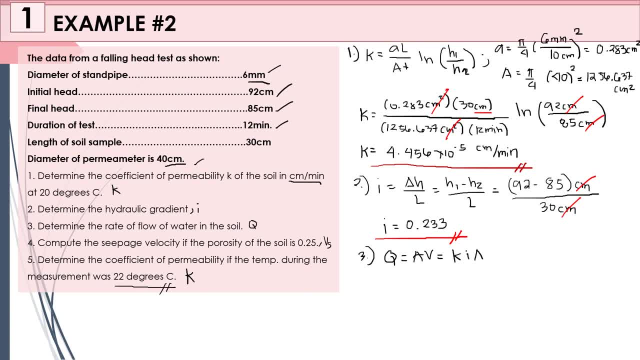 That is K times I times A. That is your coefficient. So that is your coefficient of permeability times your hydraulic gradient times your area. Okay, Therefore, Q is equals to 4.456 times 10, raised to negative 5 centimeter per minute, times your I. 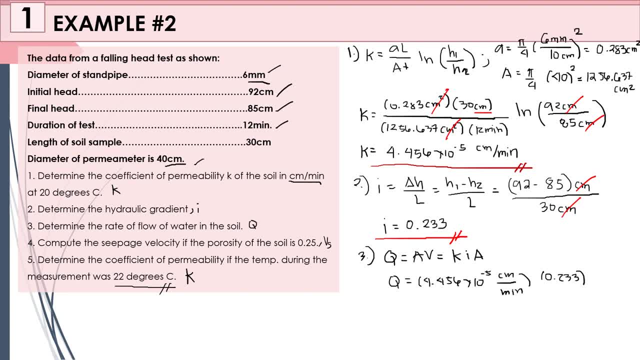 which is 0.233 times the area Anong area natin, That is 1,256.637.. So baba na lang kasi di ka siya, And that is centimeter squared, So hindi naman strict yung problem. 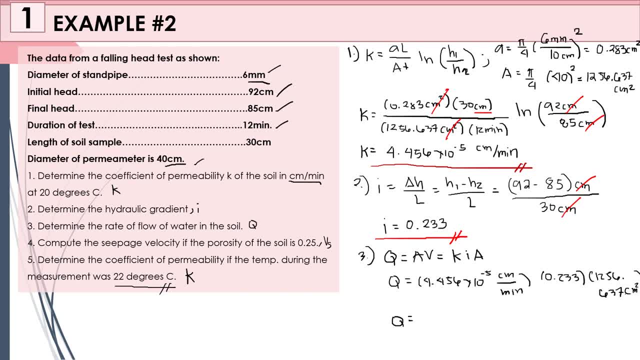 Ibig sabihin in centimeters per minute. pa rin tayo, Okay, And I think the value of that is 0.013.. Centimeters times centimeter squared, That is equivalent to cubic centimeter over minute, And that is our answer. 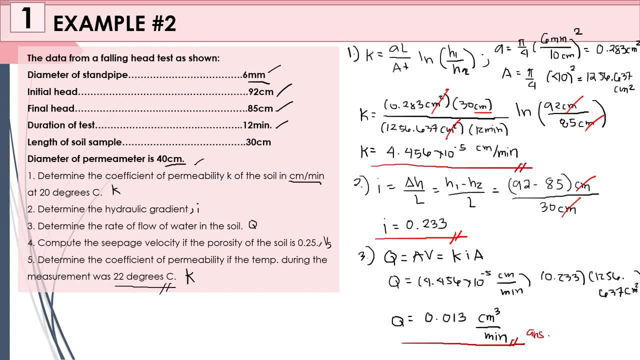 Okay, Last is number four. O dito na tayo. Number four is that solve for the value of your coefficient of permeability, if K is I mean if the temperature is 22 degrees Celsius. So ito hindi ko pala ito nabasa kanina during our formulas. 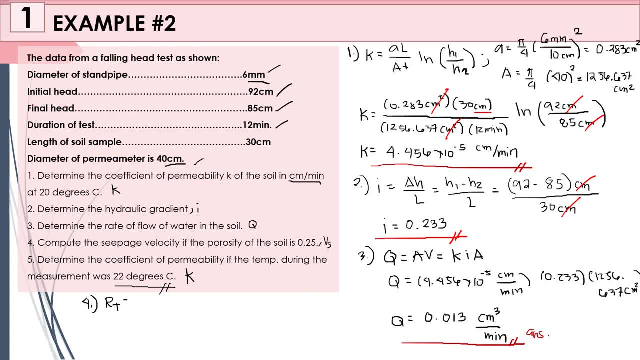 Pero balikan nyo na lang yung slide na yun Kasi meron doon nakalagay that RT is equivalent to 2.4.. 42 minus 0.475 ln of T. Okay, Kasi, kahit magbigay siya ng situation na na-measure yung coefficient of permeability natin into different temperature. 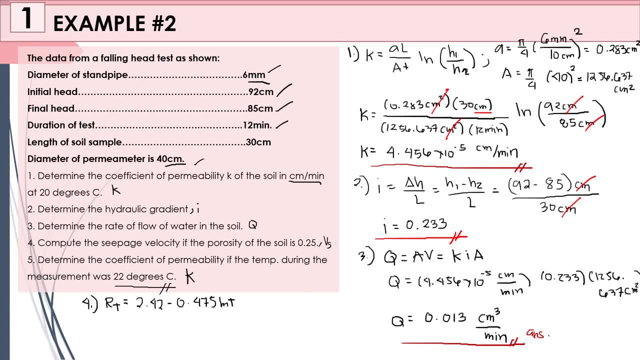 take note that yung K na pinag-uusapan natin dito is expressed in 20 degrees Celsius. Okay, So parang ang mangyayari nito is: ibabalik, at ibabalik pa rin natin siya sa 20 degrees. 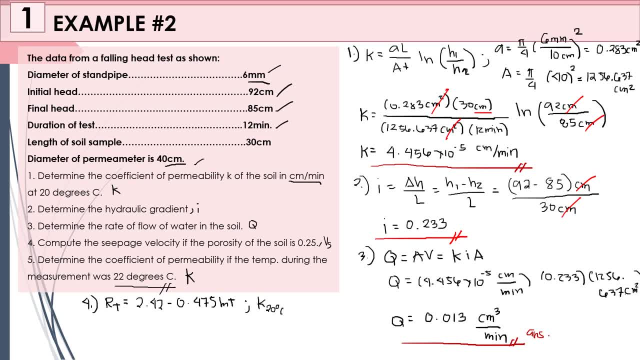 Okay, And the formula of a coefficient of permeability in 20 degrees, that is K times your RT, Okay. So paano natin gagawin ito? So solve muna natin yung RT. So RT is equals to 2.42 minus 0.475 ln of yung temperature na binigay ng situation, which is 22.. 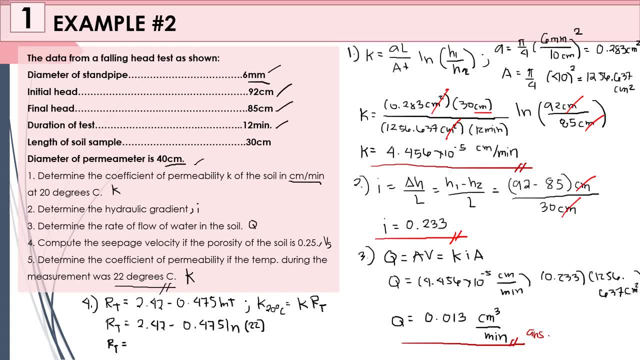 Sige, Okay Solve, And I think the value of that one is 0.952.. Okay, So, to get the value of our coefficient of permeability at 20 degrees, relate lang natin siya sa 22 degrees. 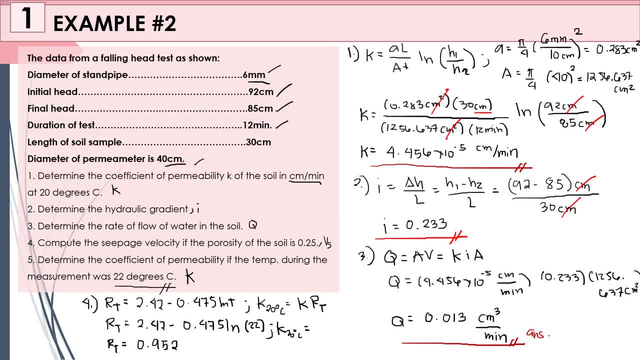 That is the value of our K times PT. So siguro store nyo na lang ito kay A, kasi hindi na ka siya sa aking solution. So lagyan ko na lang ng A dito Para alam nyo kung saan yan ang galing. 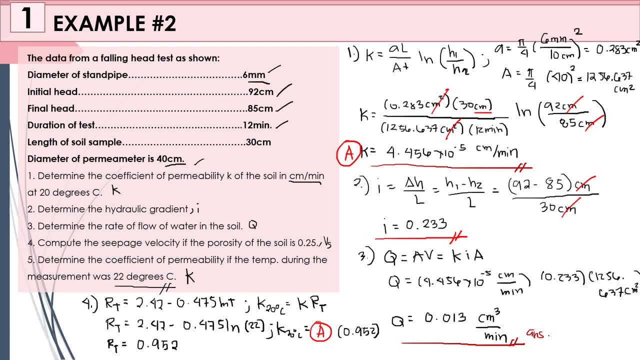 Times 0.952.. So kindly check if the value of that one is equivalent to 4.242 times 10, raised to negative 5.. And what will be the unit? the matik, that is, centimeter per minute, The same as ang nakuha natin kanina sa first. 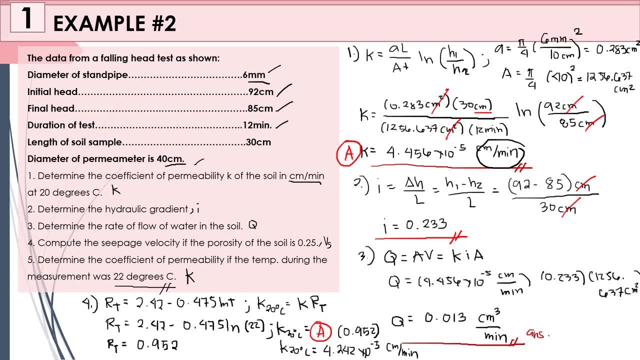 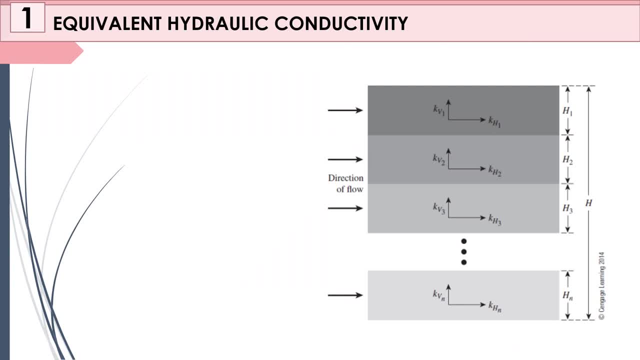 Problem, And that is our answers for four problems. Okay, So, pag-uusapan naman natin ngayon yung equivalent hydraulic conductivity. Okay So we have horizontal and vertical, So let us talk about the horizontal muna. 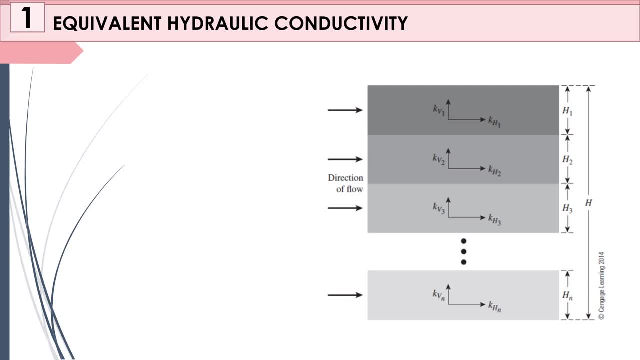 So this diagram tells us that this hydraulic conductivity is horizontal. So you have your H1, H2, H3, and Hn- that is the height of your soil specimen, And you have here the direction of flow. dito pumapasok yung ating fluid. 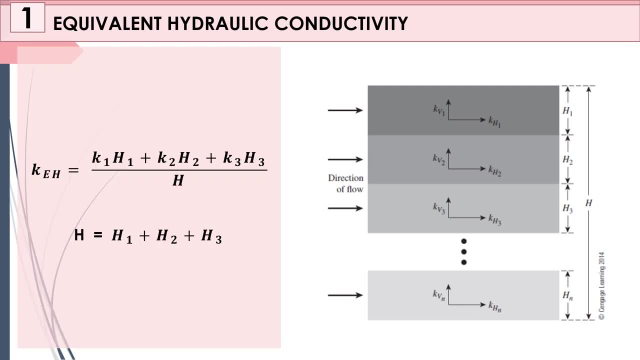 Okay, So this is the formula for your horizontal. so lagyan natin dito: Ito ay horizontal, So lagyan natin dito: Okay, So this is the formula for your horizontal, So lagyan natin dito. 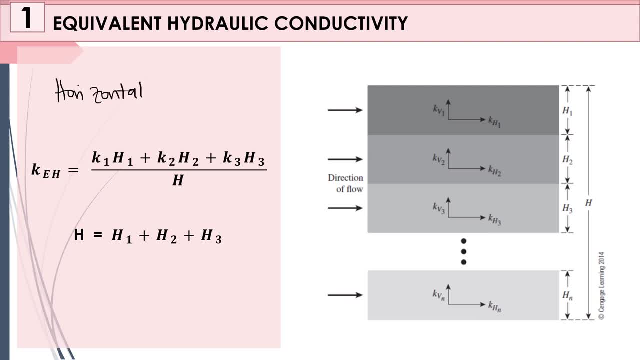 Okay, So this is the formula for your horizontal. So lagyan natin dito. Okay, Okay, So dito na lagyan natin Horizontal equivalent hydraulic conductivity. So ganyan lang yung ilalagay natin. 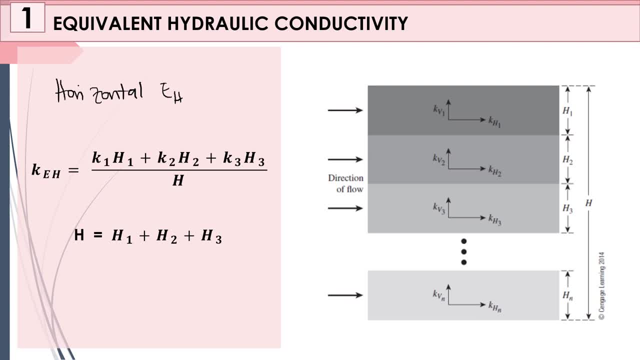 So mam, kaya po ba siya tinawag na horizontal equivalent hydraulic conductivity, kasi yung flow po ng fluid is horizontal, siya pumapasok. Ganun po ba yung concept nyan? The answer is no Okay. 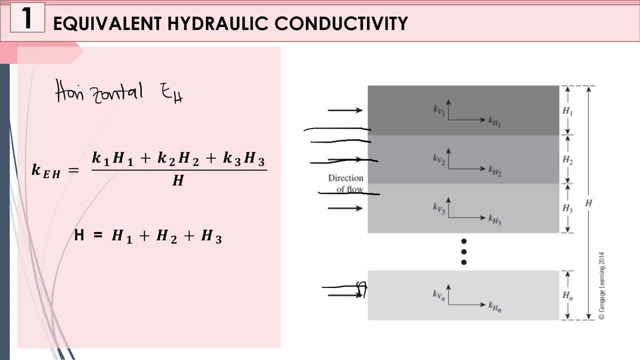 It doesn't mean na horizontal yung pangalan ng diagram na ito. I mean horizontal equivalent conductivity. hindi ibig sabihin na horizontal sya. ibig sabihin ang flow ng fluid natin is also horizontal. Mali yun, Okay. 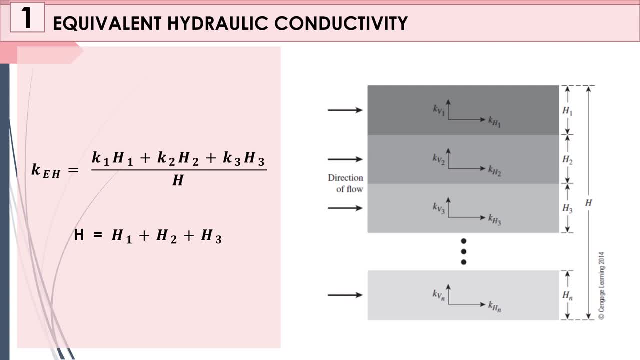 So tinatawag natin tong horizontal equivalent hydraulic conductivity when, okay, when, the fluid flow is parallel to the soil layers. Okay, So ano bang ibig sabihin ng parallel? Ibig sabihin go with the flow sya. 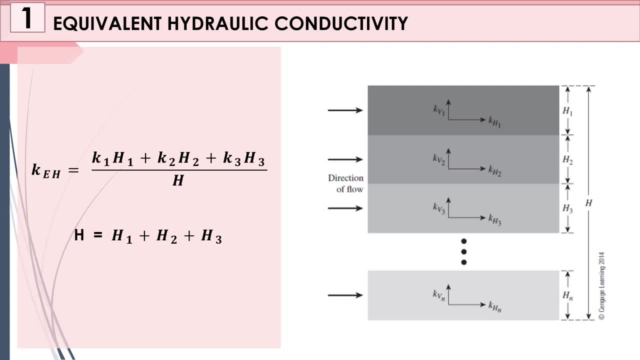 sa layers natin. Ano ba yung layers ng soil natin? Okay Ito, This is the first layer of our soil, which is H1.. This is the second layer, H2, and the third layer, H3, so on, and 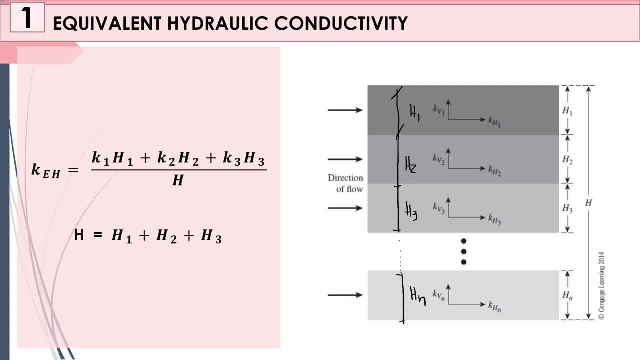 so forth. This is your Hn, So if this is your soil sample, okay, if yung tubig natin or yung fluid din, yung is pumapasok sya layer per layer sa ating soil, ibig sabihin, 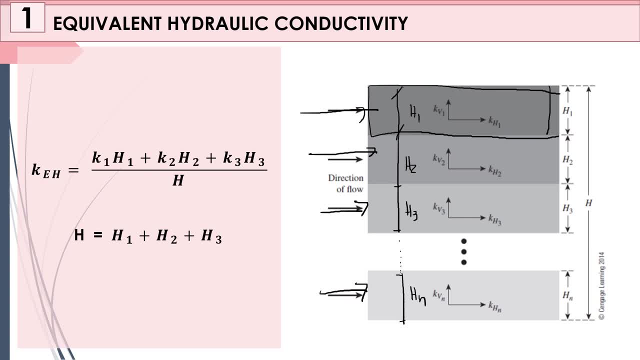 kinoconsider na natin yun as horizontal equivalent hydraulic conductivity. Okay, Ibig sabihin, yung fluid flow natin is with respect to the soil layer. Tanda nyo yan ha, If your soil or if the direction of your flow is. 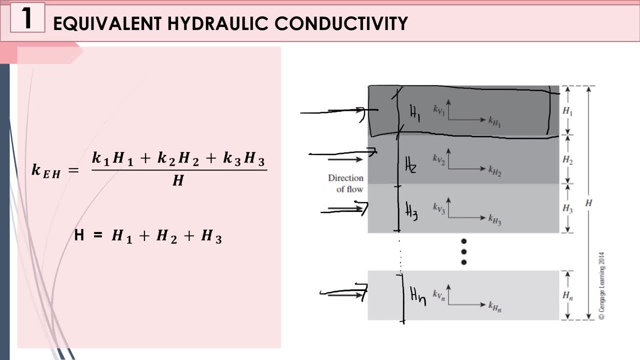 parallel to your soil layer, that is, your horizontal equivalent hydraulic conductivity. Okay, And we have a formula for that. No, That is equals to K1H1 plus K2H2 plus K3H3 over H. But take note. 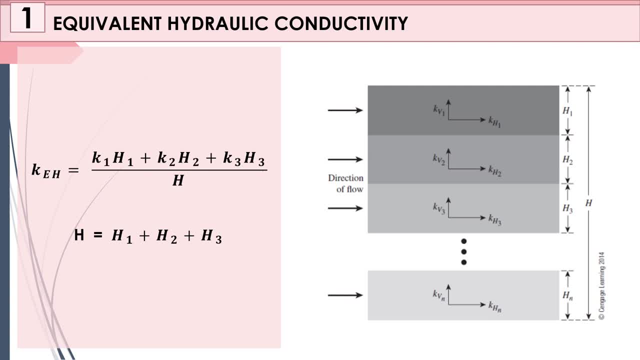 no, Kapag marami tayong layer hindi yan sya hanggang H3 lang. No, Idat-dat-dat natin yan KNH3.. Where your K is your coefficient of permeability and your H here is the height of the layer. 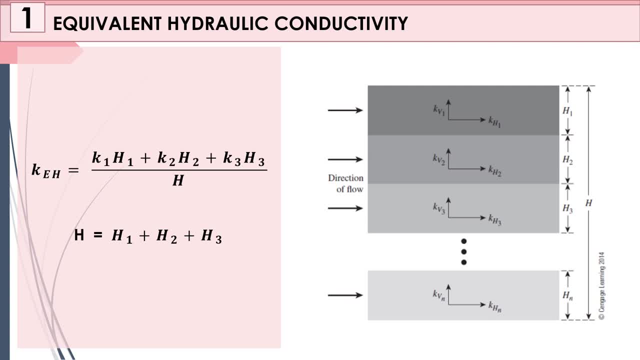 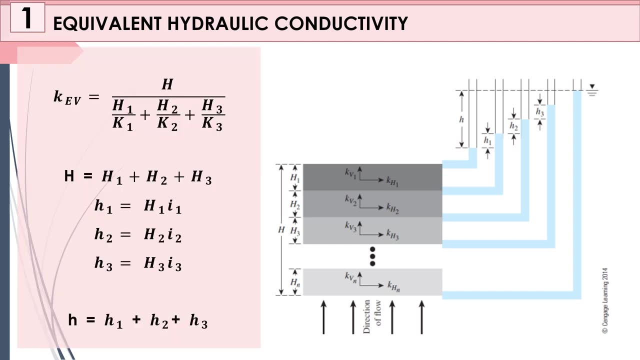 So over H, so yung H natin as the denominator. that is the sum of all the layers, That is H1 plus H2 plus H3.. Okay, So we also have this one. Okay, And ito naman yung inyong vertical. 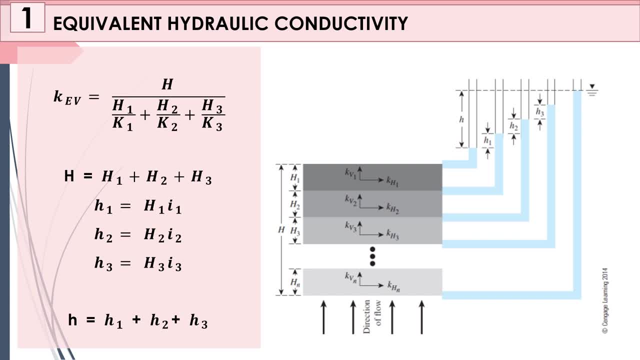 equivalent for hydraulic conductivity. So we have here your piezometers. No, Yan pumapasok yung ating tubig na nananggaling sa soil. As you can see, yung direction of flow natin is galing sa baba. 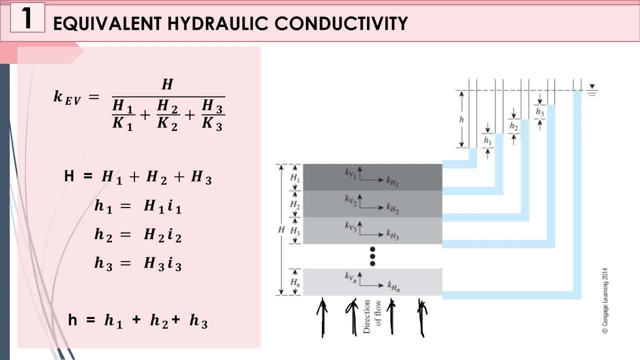 Okay, That is the direction of your flow. So how you have here your H, your H1, your H2 and H3, that is the difference between the height of the water inside our piezometer. Okay, So pag sinabi naman natin. 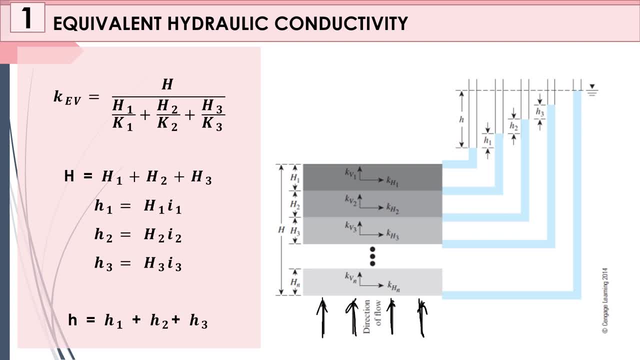 yung vertical equivalent hydraulic conductivity, yung flow nito is crosses yung ating soil layer, No, Or, para mas maging madali, siguro yung pagkakaintindi natin: Okay Kung kanina, okay Kung kanina, so horizontal. 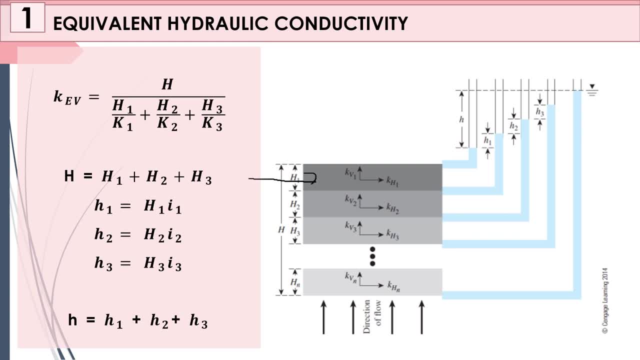 matatawag natin yung siyang horizontal if yung direction ng flow natin is parallel to the soil layer. Ngayon naman, matatawag natin siyang vertical if yung direction of flow natin is perpendicular to our soil layer. 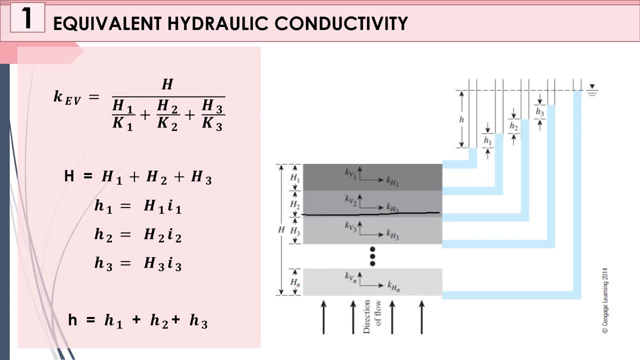 Can you see that it's perpendicular. This is the layer per layer of our soil, Okay, And this is the direction of our flow, Which is: this is perpendicular: Nuggets, Nuggets. Okay, So we have a formula for your vertical equivalent hydraulic conductivity. 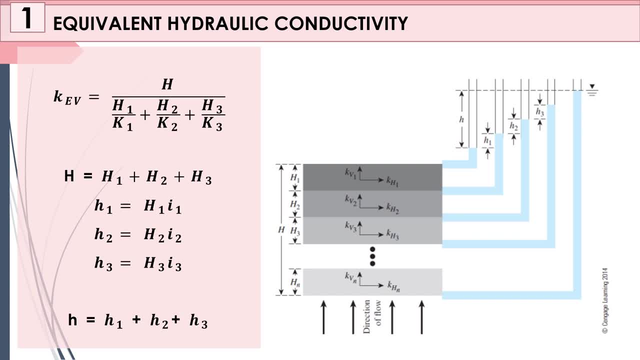 that would be H1 over K1, plus H2 over K2, plus H3 over K3.. It's still easy to memorize right Where your H1 there. that would be H1 times I1.. What is our I? 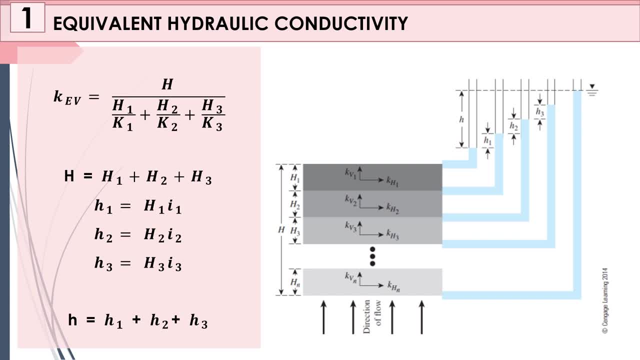 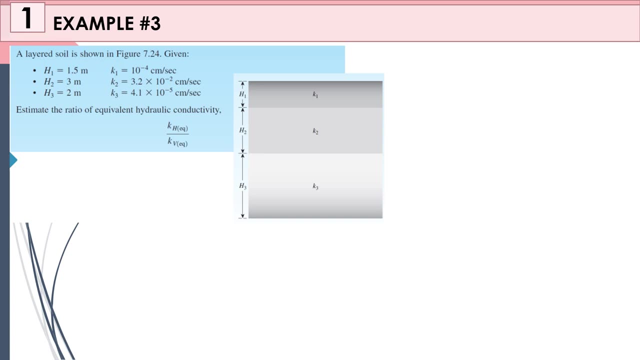 That is your hydraulic gradient. So this is the difference between this height and this height. That is our I. Okay, So on and so forth. So let us try to understand how that would happen. Okay, So it says: here we have a layered soil given. 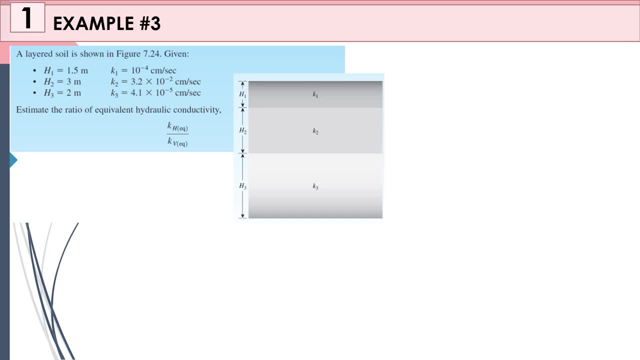 So you have H1, H2, and H3, as well as for your K1, K2, and K3.. So let us try to estimate the value of your hydraulic conductivity. So when we say ratio, that is between KH over KV. 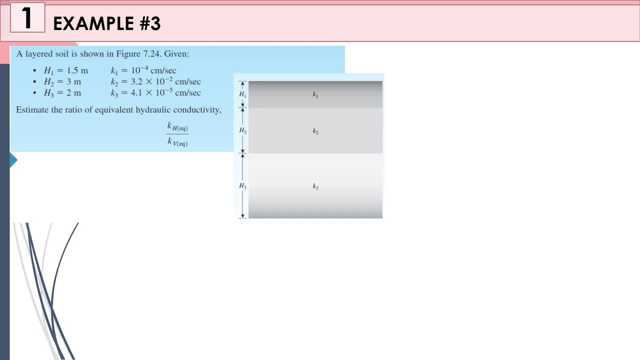 Okay, Take it. So before we get the ratio, we need to get the value of KH and the value of KV. So let us write down their properties first. It says here: H1 is 1.5 meters, H2 is 3 meters. 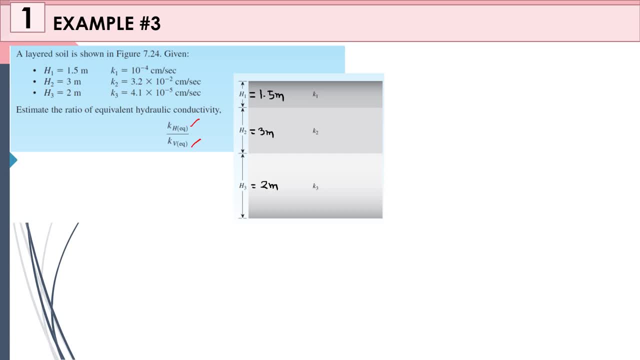 And H3 is 2 meters. So let us first solve the. Let us just go here. Let us first solve the horizontal. Okay, Our horizontal formula. what is that? The formula of horizontal? Okay, So that is K1H1 plus K2H2 plus K3H3 over H. 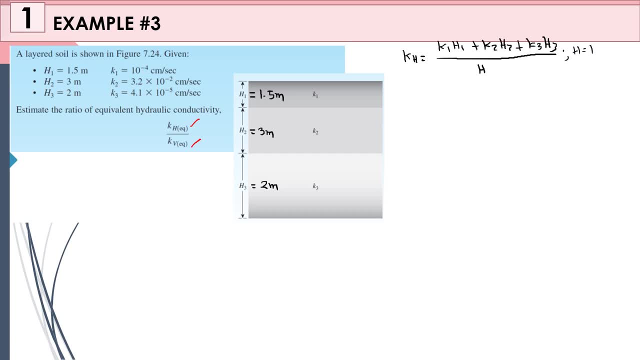 Where our H here is the sum of H1 plus H2 plus H3.. Let us first get our H here. Okay, H is equal to 1.5 plus 3 plus 2. And that is equivalent to 6.5 meters. 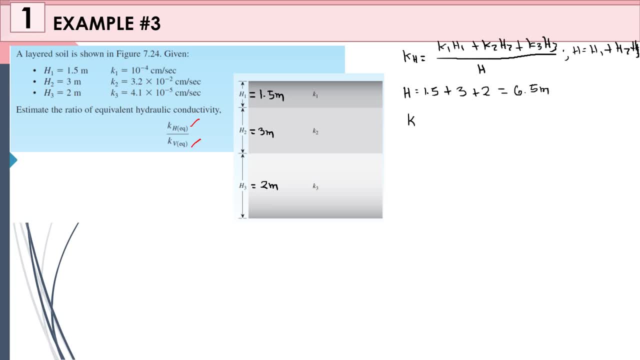 Okay, So let us just solve it, Mom. we have a question. Mom, are we not going to convert the meters to centimeters, since our coefficient of permeability is in centimeters? Actually, it is not necessary anymore, Because we can cancel it later. 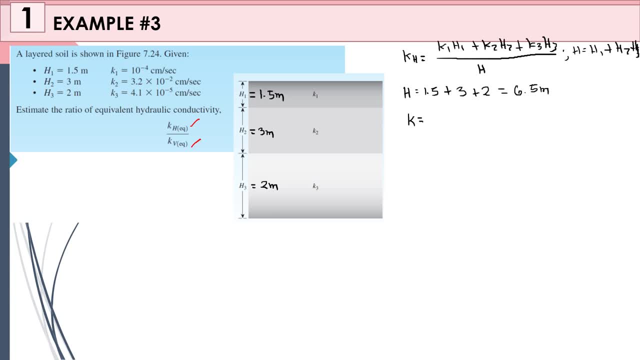 Okay, Look at this. So it says here: let us first write K1H1.. Let us write this as H K1H1.. Our K1, that is 10, raised to negative 4 centimeters per second times. what is H1?? 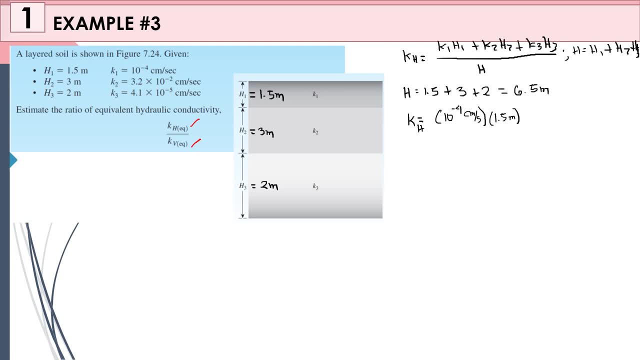 1.5 meters, Okay, Plus our K2.. That is 3.2 times 10 raised to negative 2.. I will just write C over S Times: 3 meters Plus our H3. And K3. That is 4.1 times 10 raised to negative. 5 centimeters per second times 2 meters. 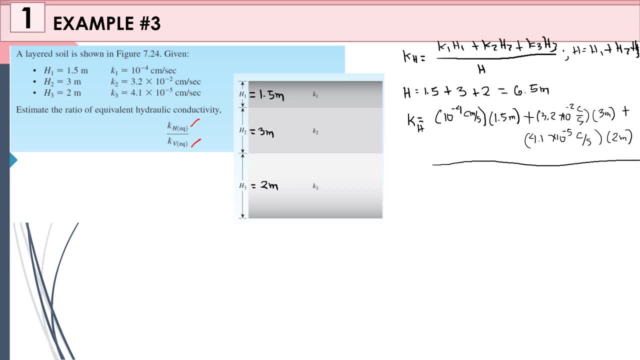 Divided by the value of our H, which is 6.5 meters. So the meters are already cancelled, Right? Yes, it is cancelled. That is just algebra: Meters, meters, meters, meters is cancelled, So what is left now is centimeters per seconds. 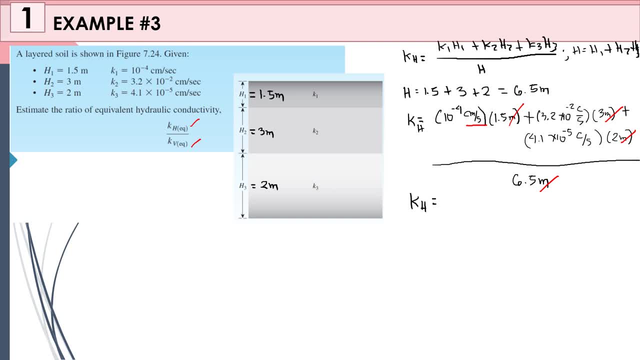 Okay, Let us compute. How many is that? Let us just check. Okay. If the value is 148.05 times 10, raised to negative 4 centimeters per seconds, Let us just check Okay. So let us try to get the value of your vertical equivalent hydraulic conductivity. 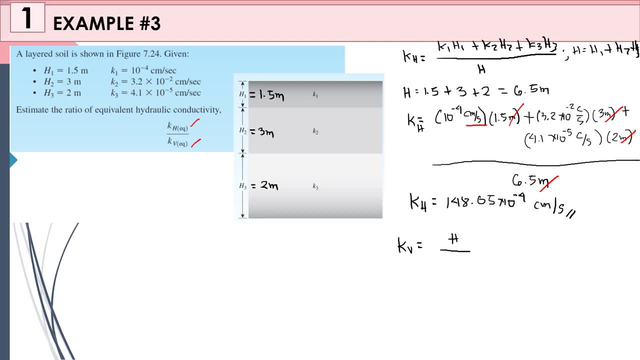 Okay, So you have your H over H1K1 plus H2K2 plus H3K3.. So this is easy. It is because there is no piezometer, No, So this is the difference between our H. 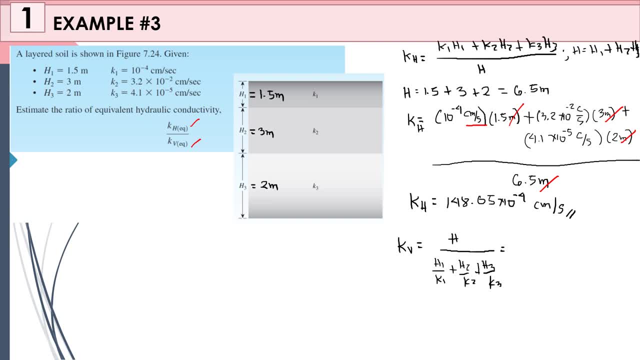 So let us just rely on this figure. So that is 6.5 meters over the value of our H1.. That is 1.5 over. I am not sure if I should write K, because it does not fit in our test. 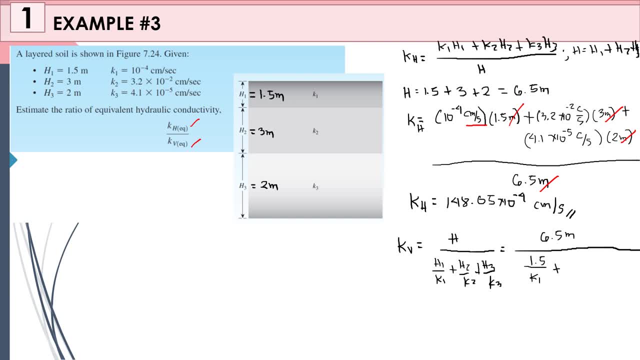 My path is so beautiful. Let us just look at the given. Okay, H2 is. I will just put the meters so that we can see the cancellation later. Okay, 1.5 meters. 3 meters over K2 plus 2 meters over K3.. 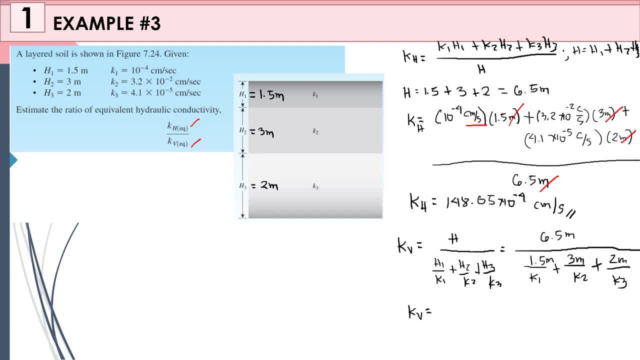 Therefore, Okay, Let us just solve this, Pause this. Let us solve this. Therefore, our KV is equivalent to 1.018 times 10, raised to negative 4 centimeters per second. We have not yet answered that. So to get the ratio of our hydraulic conductivity: 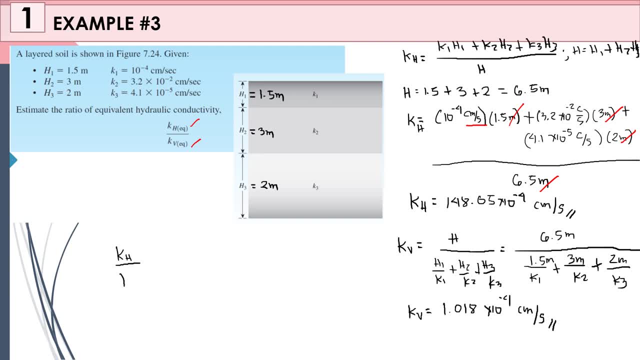 That is KH over KV. So that is 1.08.05 times 10 raised to negative 4 centimeters per second. over 1.018 times 10 raised to negative 4 centimeters per second. Unit here will be cancelled. 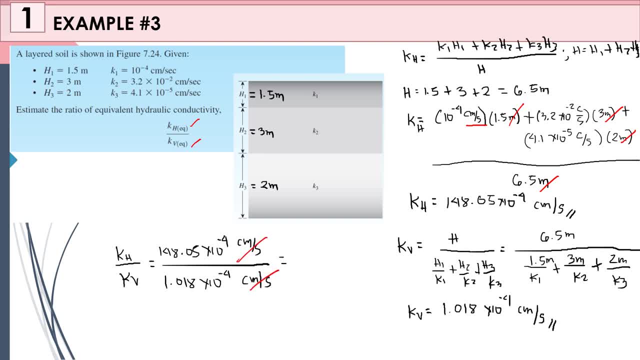 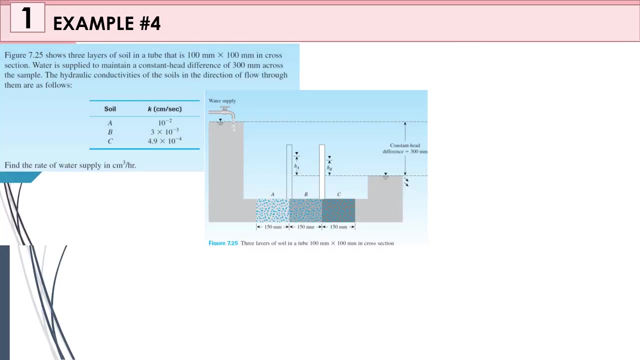 So get the value, Get the value. And I got In English, I got, And I got 145.4.. Just check if that is correct. Okay, And that is your answer for the given problem. So let us try example number 4.. 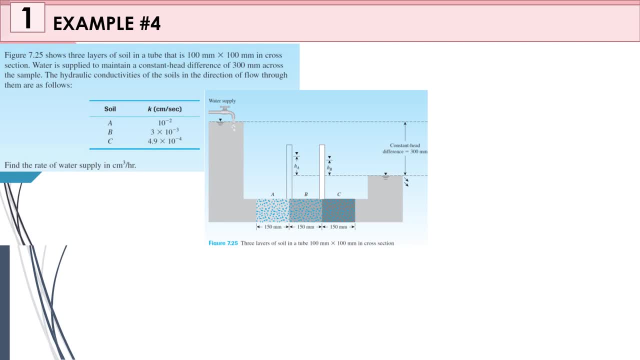 So we have here 3 layers of soil in a tube that is 100 mm, 100 mm by 100 mm, So water is supplied to maintain the constant head difference of 300 mm. So the hydraulic conductivity of the soil direction, of the flow through, given in the data, 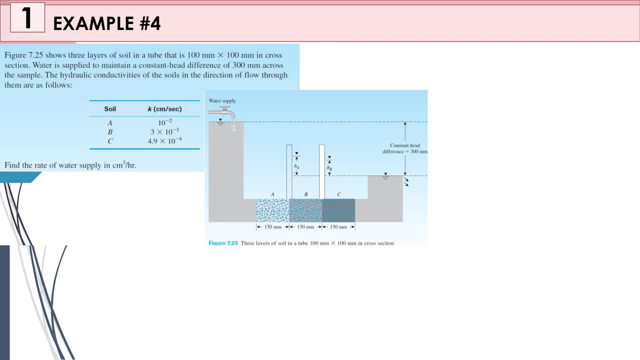 So you have ABC, that is your K, or your hydraulic conductivity, that is in centimeter per second. So we have soil A, soil B and soil C. Okay, The length per soil is 150 mm. So our height, or your constant height, okay, that is 300 mm. 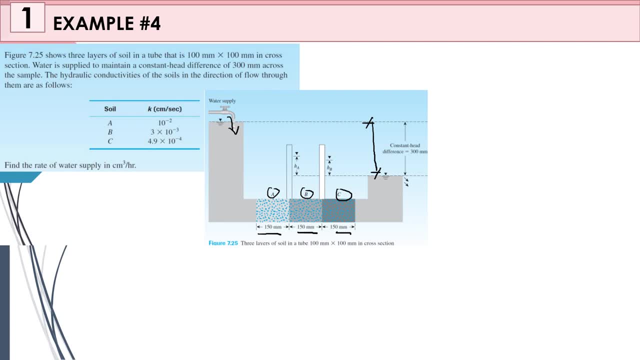 So this is the inlet, That is where our soil enters and here it is discharged. So constant head does not change our elevation, It is still 100.. So the area of our soil in tube that is 100 by 100. 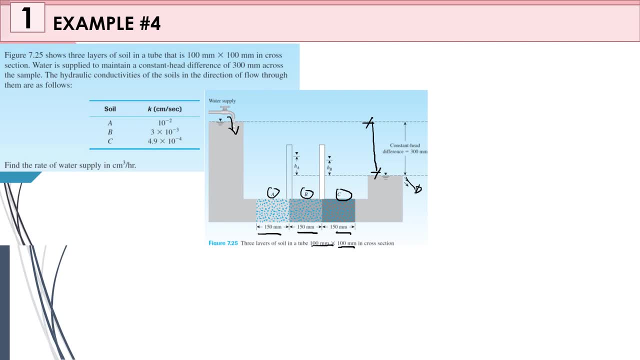 So what we are going to look for now will be the rate of water supply in cubic centimeter per hour. Okay, So that is where we will have a hard time. It is because the unit is different, because we have mm and centimeter. 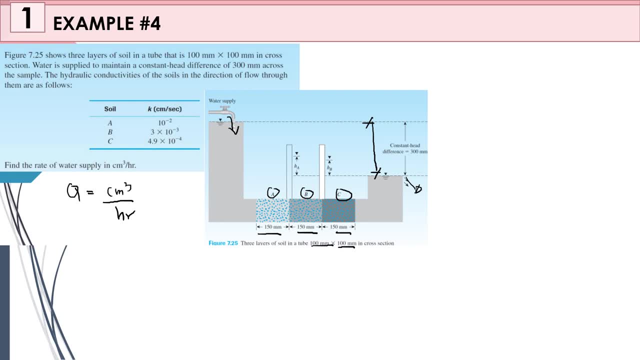 But, regardless, that is easy. Okay, So what we are going to use here is to solve the value of K. Mom, it is easy. We will just add the K of A, B and C. We will just use total. 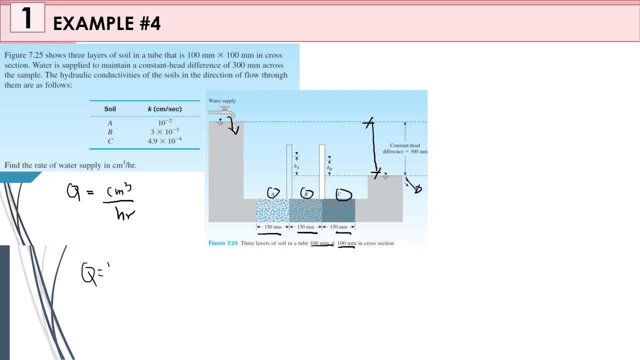 So, mom, if we get the K, that is just K, right, mom? Oh, yes, correct K. That is what we will use, because your hydraulic conductivity, your hydraulic gradient, your hydraulic gradient is H over K. Yes, H over L. 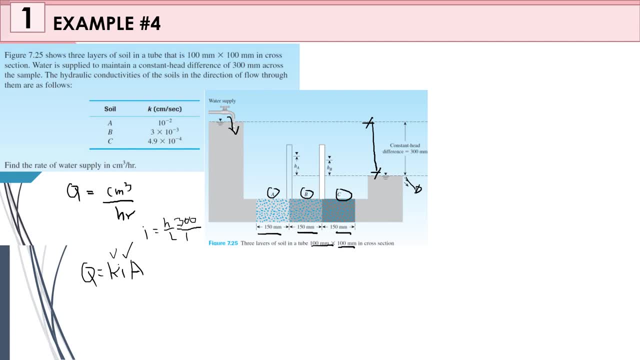 Where our H is 300 and our L is 150 times 3.. Our area was given the cross-section 100 by 100.. Yes, that is correct. Nokia will really use that. But is it correct? We will just add this. 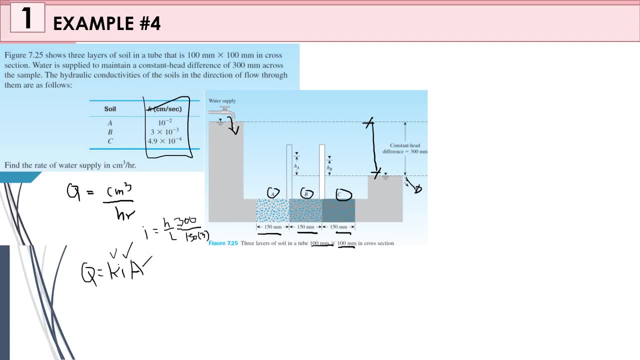 The answer is no, Because that is the coefficient of permeability per soil. That is the soil There, But how about if it already has water, or we already added water to it? it already has direction of flow. It means that our coefficient of permeability is changing. 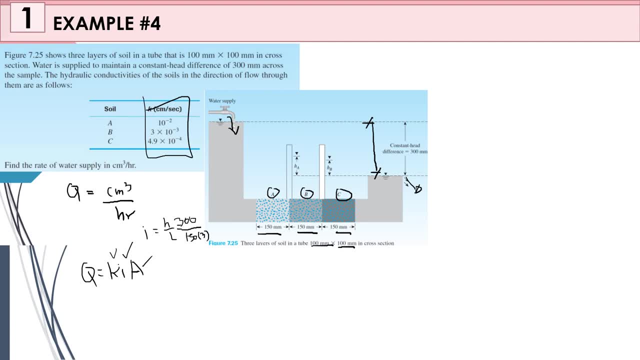 So my question now is: is that horizontal or vertical? Where did it come from? I will erase this. Where did our water come from? It came from here. right Water supply, it will flow, Flow. Oh, this is our flow here. 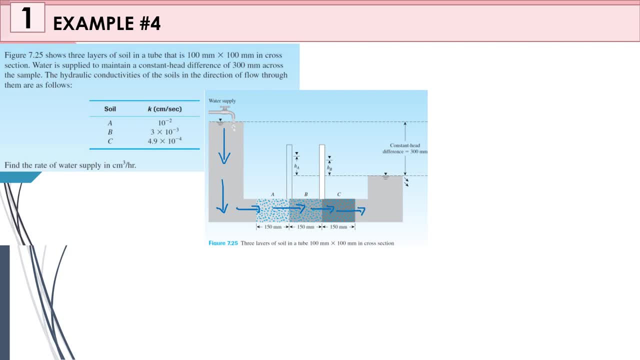 So what is that? Is that horizontal or vertical? What is the orientation of our direction of flow in our soil? Look at it. Okay, let us spill it. The answer is vertical. Okay, Again, how can we say if the equivalent hydraulic conductivity is horizontal or vertical? 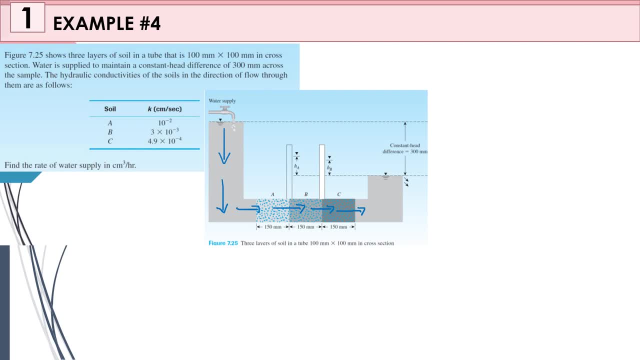 That is based on its definition. If we say horizontal conductivity, if this is your soil layer H1 and H2, the direction of your flow is parallel to your soil layer- Okay. But if the direction of your flow is perpendicular, okay. 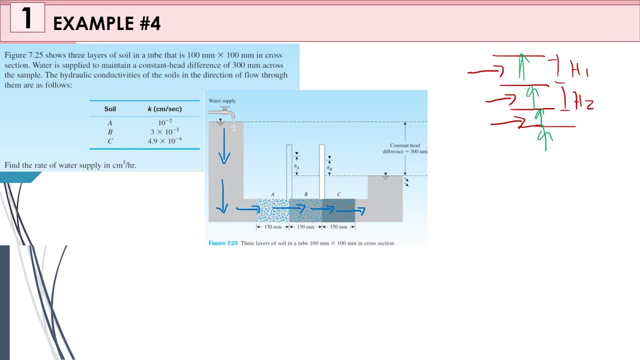 Is perpendicular to your soil layer. therefore, that is vertical. So my question now is: is this flow parallel or perpendicular? Yes, that is perpendicular. This is the layer. This is the flow. Is that parallel? No, That is perpendicular. 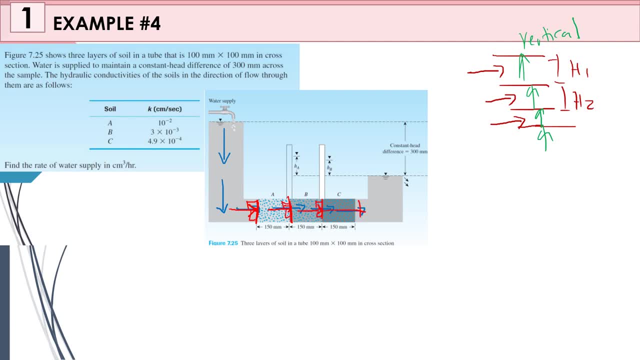 I hope I am making sense, okay, Because I can't see you right now. Okay, Okay, So it means this problem is a vertical equivalent hydraulic conductivity, Okay, Where your KV formula is H over H1 over K1, plus H2 over K2, plus H3 over K3. 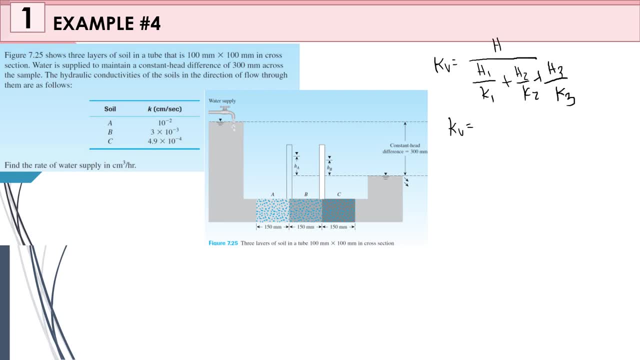 Okay, So KV is equals to the total value of your H. So this is our H: 150, 150, and 150.. So total, how much is that? 450.. Okay, Let's put MM. 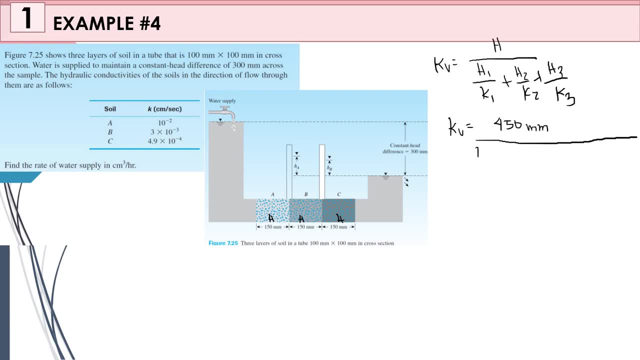 If we are not wrong later, H1,, that is 10 raised. oh, I'm wrong. H1,, that is 150 MM over 10 raised to negative 2 centimeters- Okay, Centimeter per second. Plus. H2,, that is 150 MM over 3 times 10 raised to negative 3 centimeters per second. 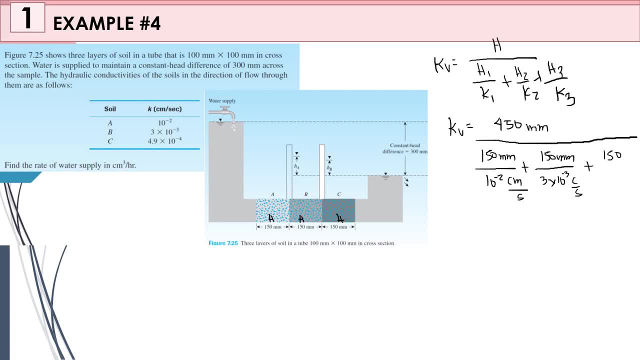 Plus H3, that is again 150 MM over our K3, that is 4.9 times 10 raised to negative 4.. So millimeters here will be canceled. What will be left is centimeters per second. So please solve the value here. 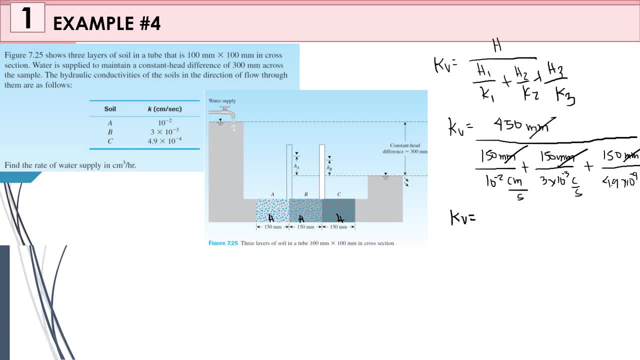 Okay, Please confirm. the value of that is 0.001213 centimeters per seconds, And that is the value of your vertical equivalent hydraulic conductivity. I'm confused. Hydraulic conductivity. Okay, So tama na yun, Nakakunin natin yung rate of flow na ninyo. 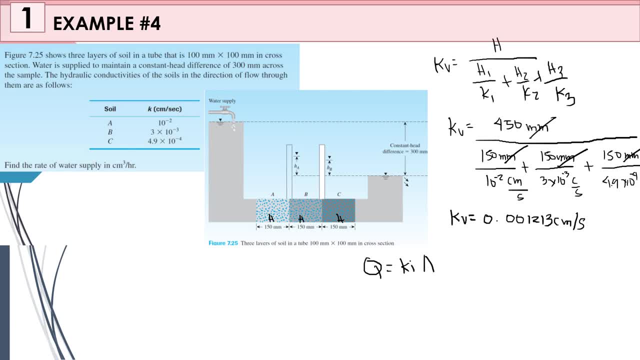 Tama, yun na Q is equal to kia. Kasi wala naman, di naman tayo binigyan ng velocity, So hindi natin pwede magamit itong ganito. Okay, So tama, yung kia natin kanina. 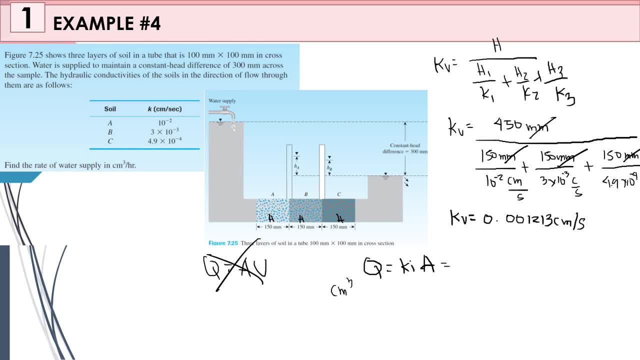 So that is that should be in cubic centimeter per hour. O dito tayo K muna K muna. 0.001213 centimeter per seconds, O seconds yan. Paano ba natin i-convert yung seconds sa R? 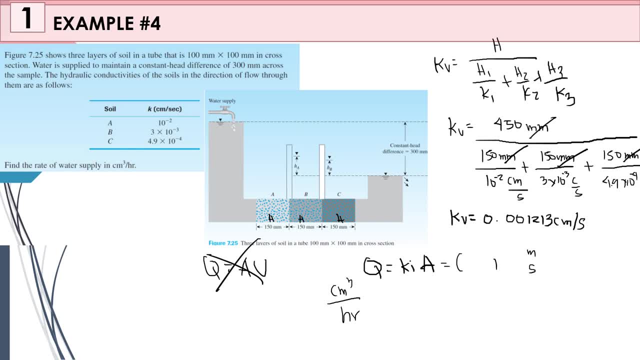 Okay, sige, ganito na lang, para hindi masyado malito yung ating nakakalito, yung ating equation, Sulat natin ulit, Okay. Okay, Q is equal to kia K-I-A. 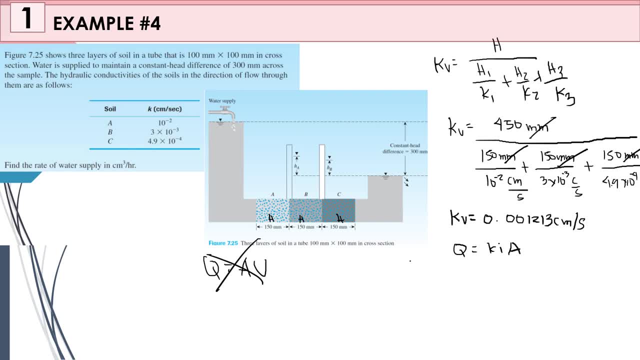 Okay So meron tayong: hindi na lang pala muna yan, Sige na lang Pati ako nalito. Okay So, meron tayong k na value na 0 point, Ano ba. 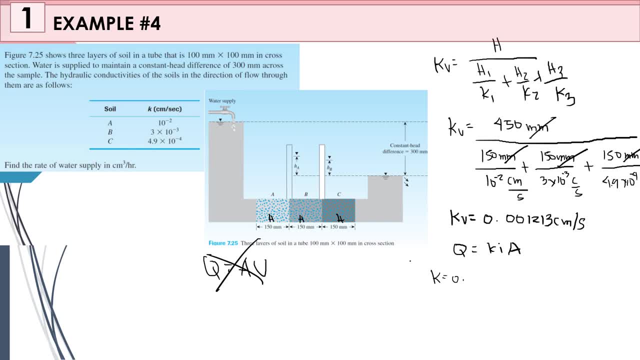 Ano bang maganda, Sige, mamaya na lang natin i-convert yung seconds to hour. No, Pwede rin naman, Sige, paano, Hindi na tayo malito. So Q is equal to 0.0101213 centimeter per seconds times your I, which is H over L. 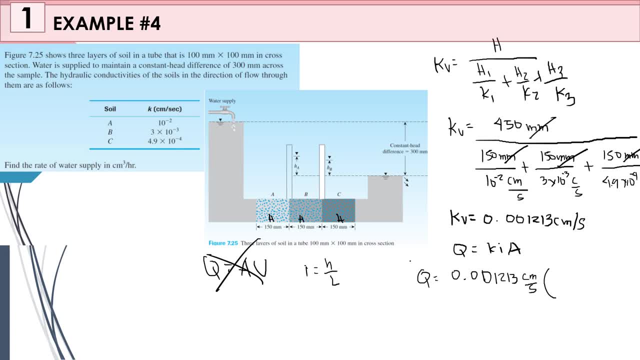 where your H, there is a constant head. therefore, walang difference between the head, Constant lang, that is 300, over the L, which is 150,, 150,, 150, that is 450.. And that is in mm Times the area. 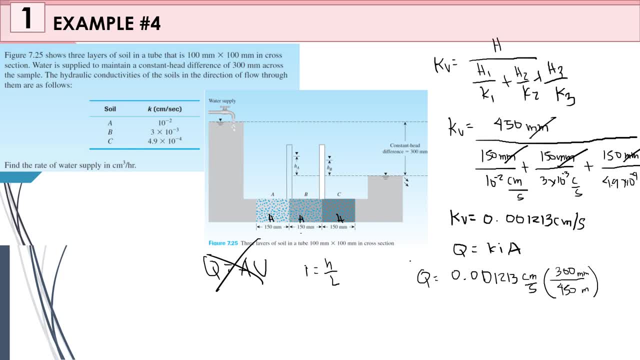 Okay, Dito ka na lang yung sa baba ilalagay, Pangit naman Sige na lang. Sa baba, na lang natin ilalagay yung area. No, Pagpasensyahan nyo lang, guys. 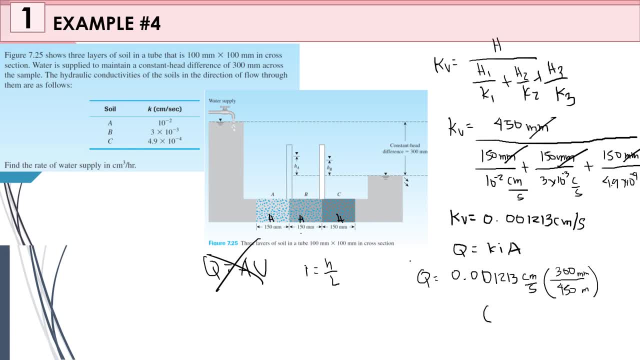 Sobrang ganda kasi ng handwriting ng inyong instructor. Okay, Area tayo, that is ano lang. base times height, So 100 times 100.. No, No, 100 times 100.. So iko-convert lang natin yan to millimeters, where i-divide natin sya ng 10.. 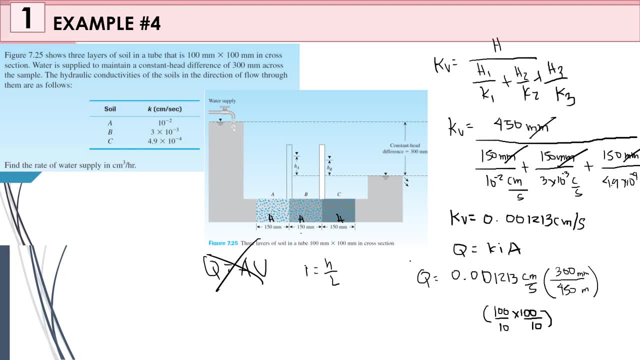 No, Para yung mm. mapalitan ng centimeters, So centimeters squared na to No, So lalabas millimeters. here will be cancelled. Nalito ba? Okay, Para di malito. balik lang sa kayo sa conversion. 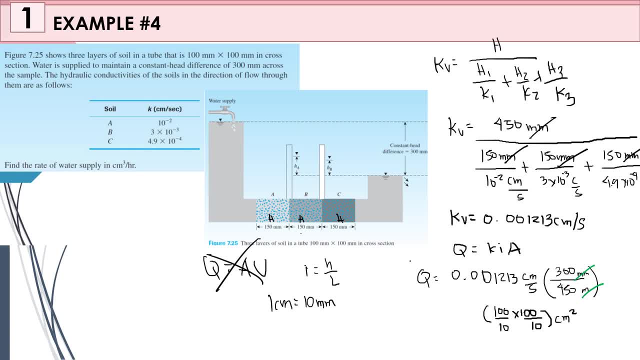 Okay, Okay, One centimeter is 10 millimeters, So kaya ako din-divide ng 10, para yung millimeters is makancel. No, Mapalitan sya ng centimeters. Okay, Nuggets, Okay. 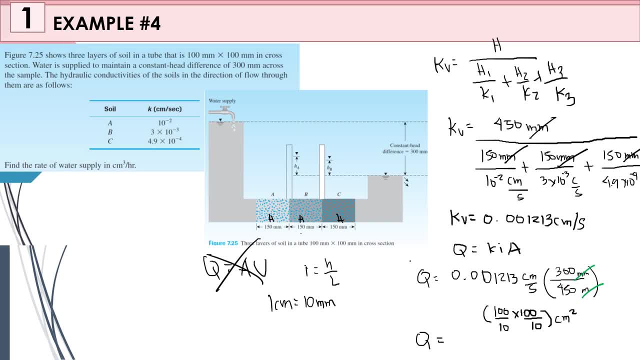 So I think how much is the value of Q here? Okay, So that is equivalent to 0.809.. And take note that is in cubic centimeters per seconds. So i-convert lang natin yung. 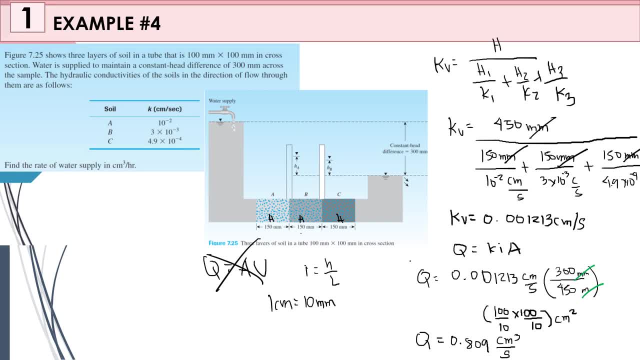 Seconds to hour. Okay, Ilan bang meron. No, So one hour ilang seconds ba meron. That is 3,600 seconds. Tama ba Ah? No, So that is 3,600 seconds. 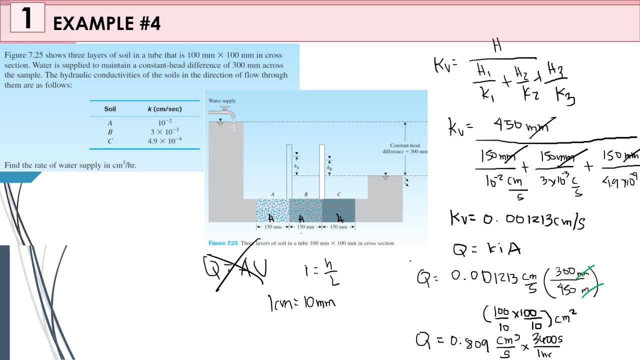 But wait, That should be 0.0809.. So seconds here will be canceled. So ilan na yung magiging answer. dapat talaga natin dito. That is 291.24 cubic centimeter per hour. 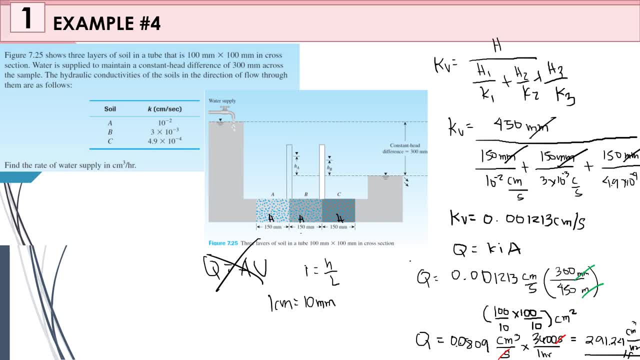 And that is our answer. I hope na-gets yan, So di n'yong masasolve tong problem. na to, If nakalimutan n'yong yung prinsipol, No, Kung nakalimutan n'yong prinsipol ng horizontal and vertical equivalent hydraulic conductivity.